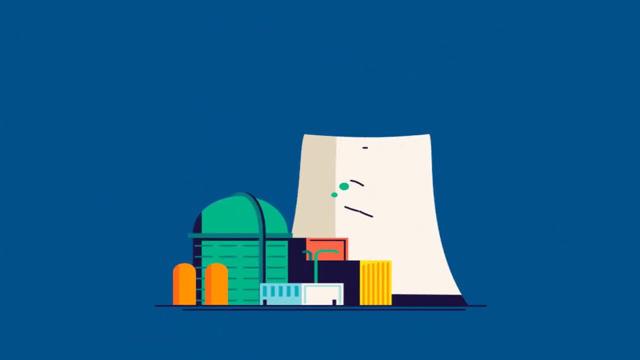 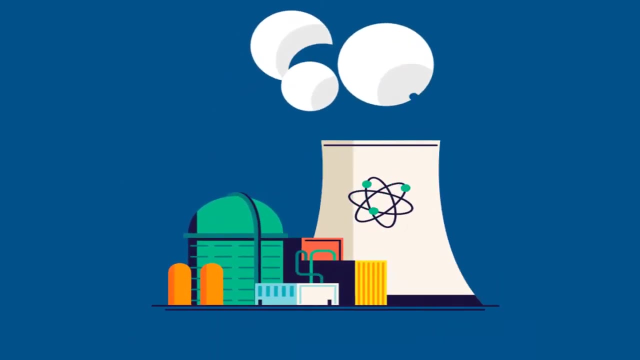 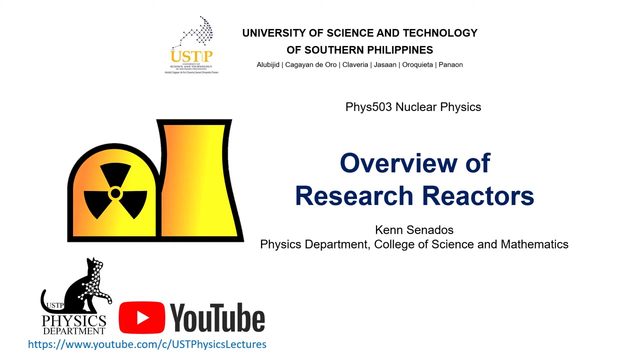 Hi, this is Physics 503, Nuclear Physics, and in this lesson we are going to have an overview of the research reactors. In this lesson we are going to discuss what a research reactor is, the applications of your research reactors, some types of your research reactors and, in the last 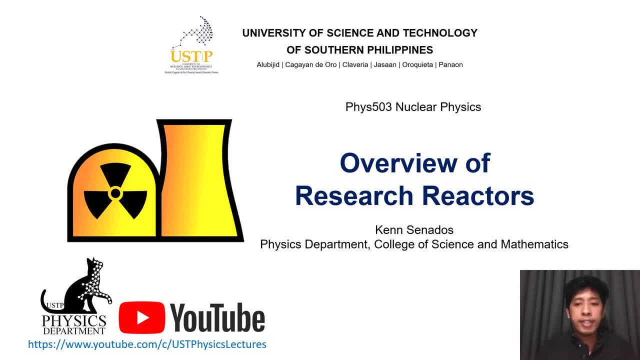 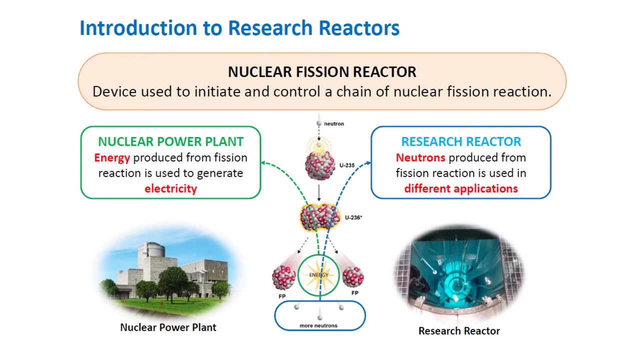 part. we're going to talk about the PRR-1 Saturn, which is the Philippines' own version of a research reactor. Your nuclear fission reactors are devices used to initiate and control a chain of nuclear fission reactions. Just for a quick review, when a stray neutron hits a heavy nuclei, like, say for: 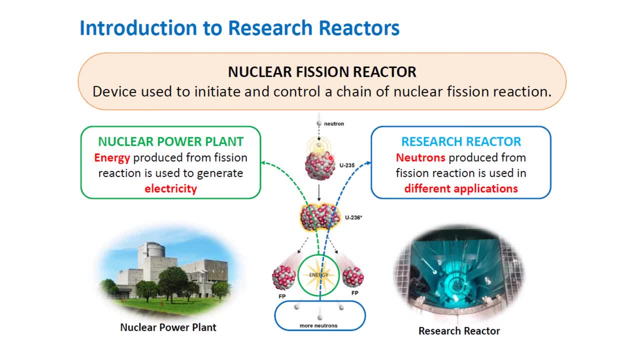 example, in this case, your uranium-235,. this neutron is absorbed, creating an unstable nuclei, your uranium-236.. This then splits into fission fragments, as this is unstable, unstable and also produces energy and more neutrons. this energy produced during the fission. 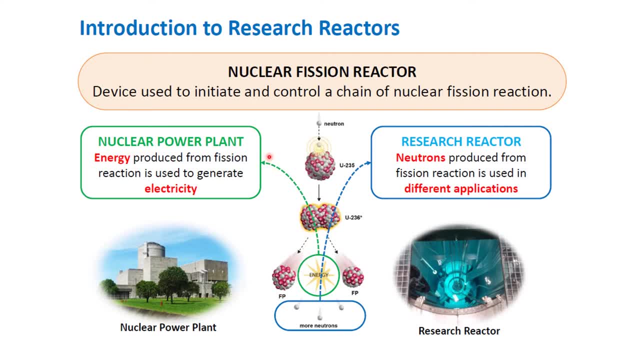 reaction is used by your nuclear power plants to produce or generate electricity. on the other hand, these neutrons, or these more neutrons that are produced after the fission reaction, is used by your research reactors in different applications. in the philippine setting we have the 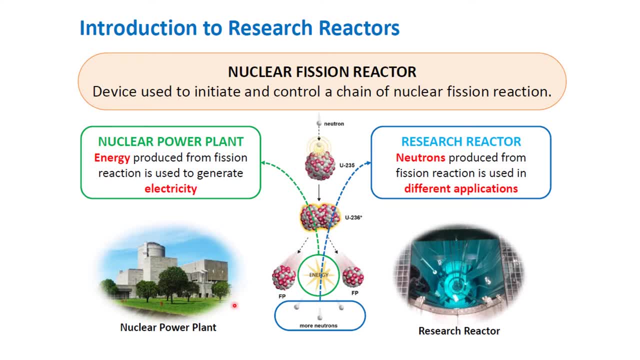 bataan nuclear power plant, which was not commissioned, and we have the PRR-1 or the philippine research reactor 1, as an example of your research reactor. your PRR-1, however, is still under shutdown. let us elaborate more. what a research? 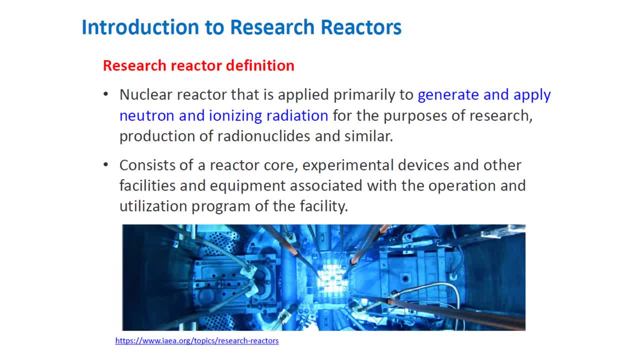 reactor is basically a nuclear reactor that is applied primarily to generate and apply neutron and ionizing radiation for the purpose of research. production of radionuclides and similar are your research reactors. it consists of a reactor core and experimental devices and other facilities and equipment. 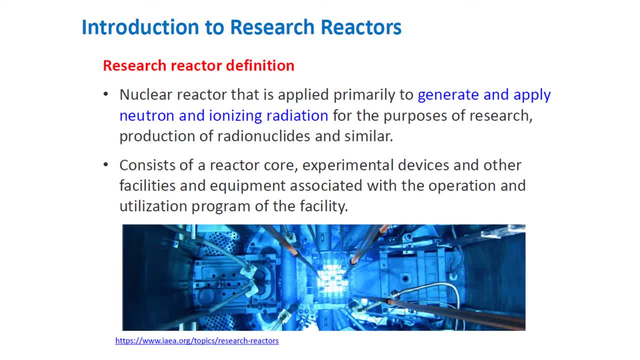 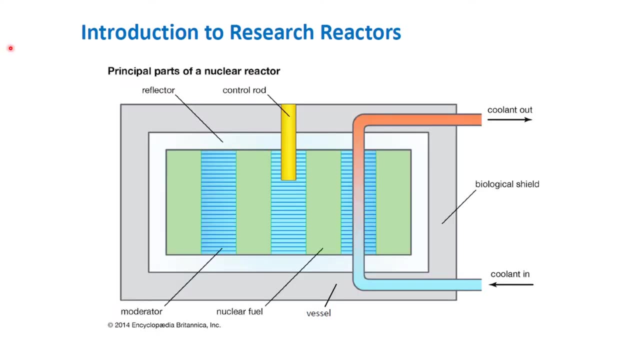 associated with the operation and utilization program of the facility. this is an example here of a research reactor taken from the IAEA. this is here is a schematic diagram of the principal parts of a nuclear reactor. now, of course, we have here your nuclear fuel, which fissions to produce these? 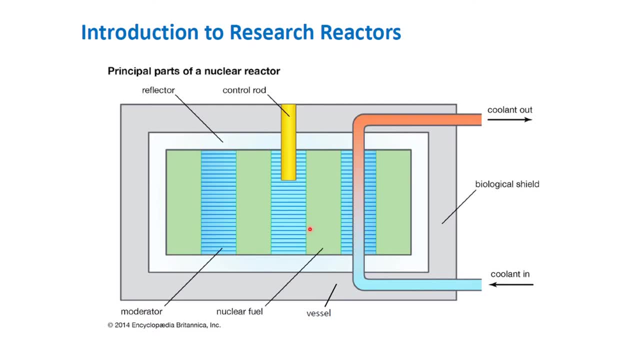 neutrons. also, you have here your moderator, a material which slows down neutrons so that more fission can occur in the fuel. remember that what we want here are thermal neutrons. you also have your reflector, this one here, which minimizes the number of neutrons that are. 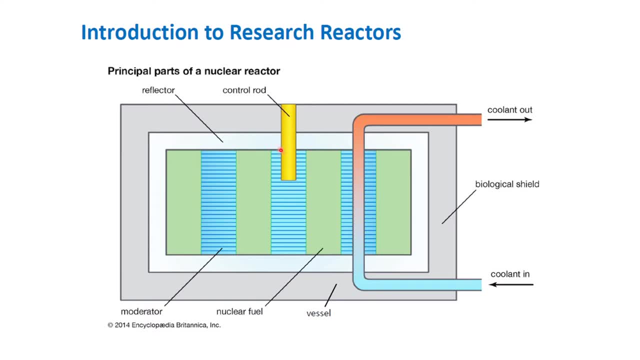 leaking out of the core, and we have the control rod which helps control the neutron population in the core and, of course, the vessel which contains all the components. now, remember that heat is also produced in the fission process, and there should be a way in which heat is removed, which is here provided by the 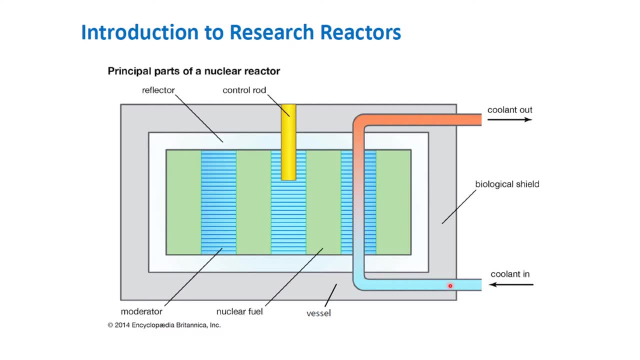 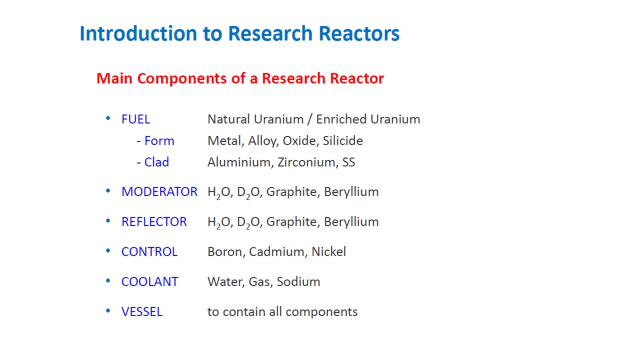 coolant. in this case, your coolant comes in and goes into a loop, taking out heat out of your core. these are other information about the main components of a research reactor. for the fuel, it can either be natural uranium or enriched uranium, and the main difference between the fuel of a nuclear power reactor and a research reactor is 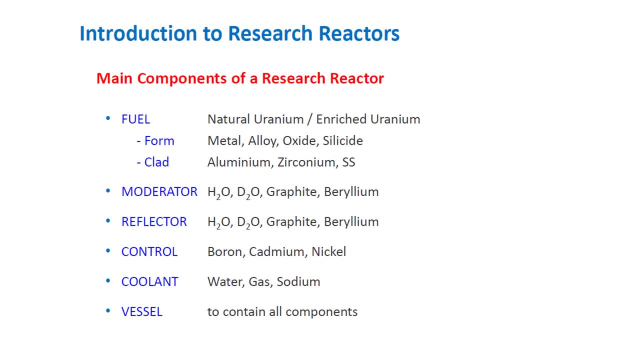 that for your research reactor, your uranium can be enriched above 20 percent. in terms of form, it can either be metal form, alloy oxide or silicide, and for the cladding you can use aluminum, zirconium or stainless steel. for example, in your philippine research reactor one 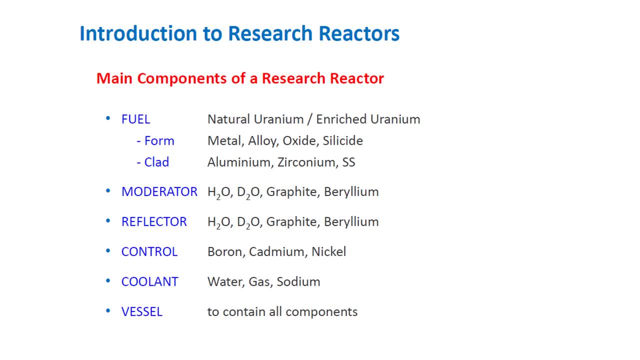 fuel is a uranium zirconium hydride fuel for the moderators. you can either use your light water or your heavy water, graphite and beryllium- the same materials are used as reflector in your research reactor and you can use any com, any combination. 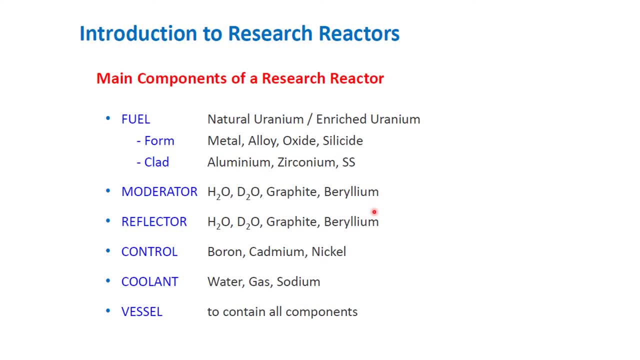 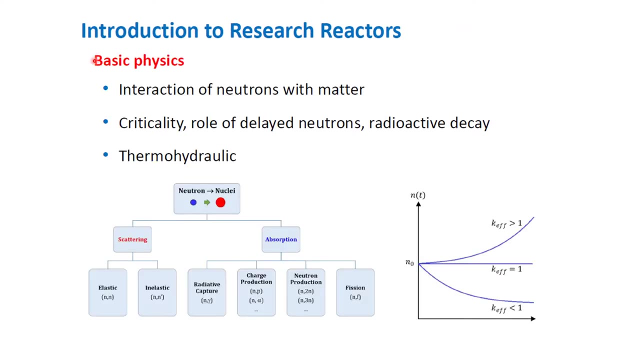 of both. for the control rods you can use boron, cadmium and nickel, and for the coolant you can use water, gas or sodium and, of course, your vessel. it contains all of the components here. the basic physics involved in your research reactors are the same physics that we see in your nuclear power reactors. 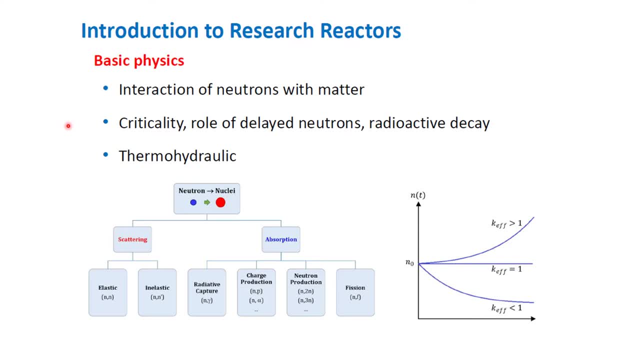 this includes your interaction of neutrons with matter, the criticality role of the late neutrons, radioactive decay and, of course, your thermo hydraulic. in. here is your critical criticality draft, or your critical criticality graph, wherein this is the state in which a nuclear chain reaction. 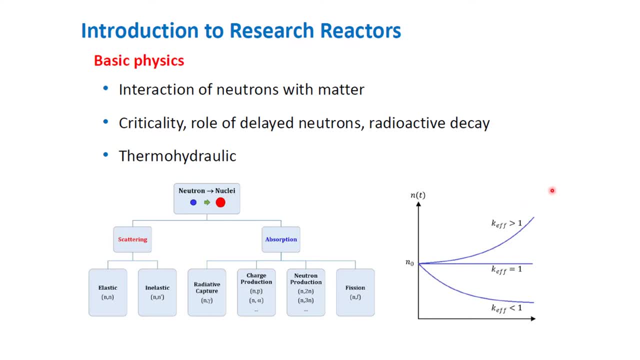 is self-sustaining. that is when your criticality graph is self-sustaining, when your activity is zero. So what we have here, your K effective. this is the effective neutron multiplication factor and this is the unit of measurement of your criticality. 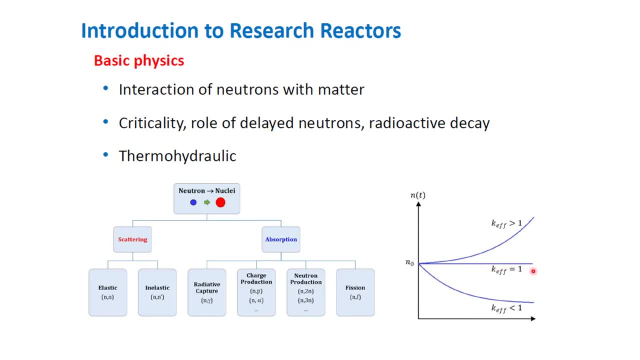 What we always want is when your criticality is equal to one, which is your critical environment. Your K effective that's less than two one is what you call your subcritical environment, and your K effective that's greater than one is your supercritical environment. 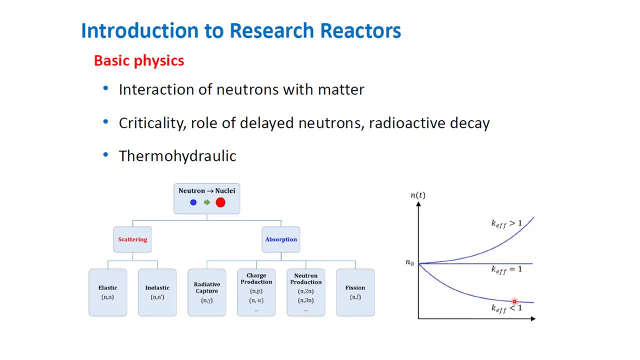 Your K effective that's less than one is when there are lesser neutrons that are produced in your fission reaction, and when your K effective is greater than one. this is when you have more neutrons that are produced during your fission reaction. 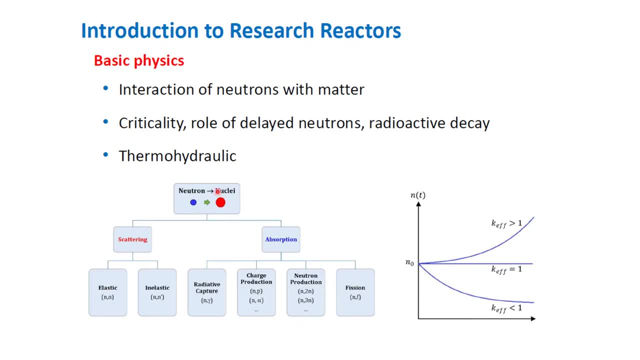 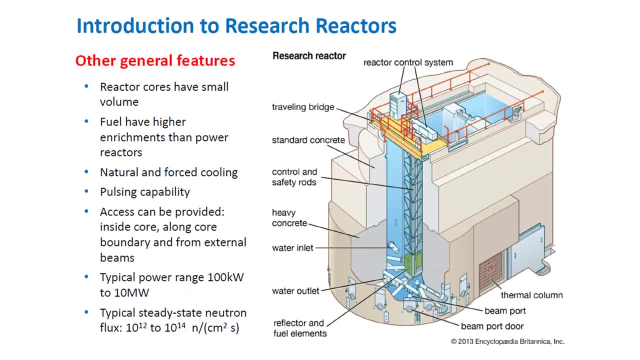 So these things here are still involved in your research reactors. Same with neutrons. So these things here are still involved in your nuclear power reactors. These are other general features of your research reactors. Your research reactors have pores that have smaller volume, typically because your fuel 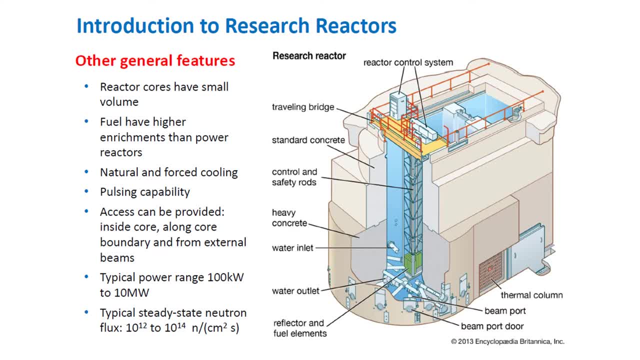 have higher enrichment than your power reactors, And for low-powered research reactors, natural convection is enough for heat to flow out of your core. But for low-powered research reactors, natural convection is enough for heat to flow out of your core, But for high-powered research reactors we should have your forced cooling. 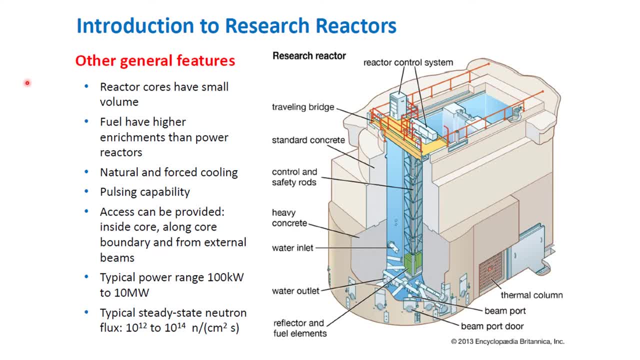 Your research reactors also has pulsing capability, wherein you can produce short bursts of energy, And, unlike your power reactors, your research reactor can provide access inside a core, along the core boundary and from external beams. Typically, the power range for your research reactors is around 100 kilowatts. 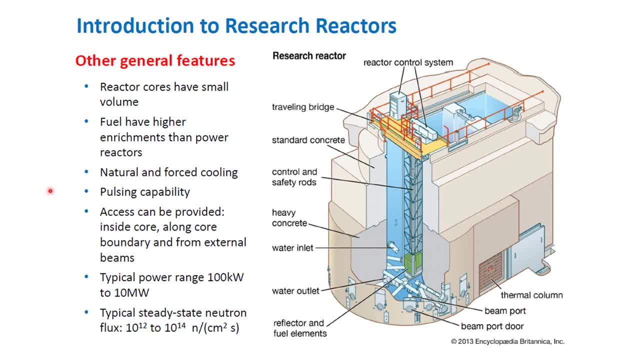 or 10 megawatts and it has a typical steady-state neutron flux of around 10 to the 12 to 10 to the 14 neutron per centimeter-squared-seconds. This is here is a schematic diagram of an example of a research reactor. 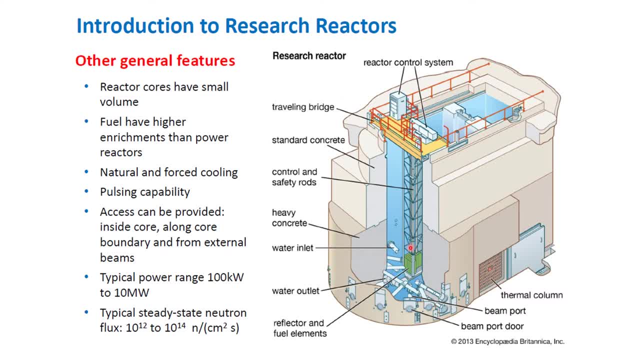 Of course you have here your reactor core, and then you also, which also contains your reflector and fuel elements, its output reactor connector used as a component itself, and then you have your water inlet and water outlet for cooling, and then you have here a heavy 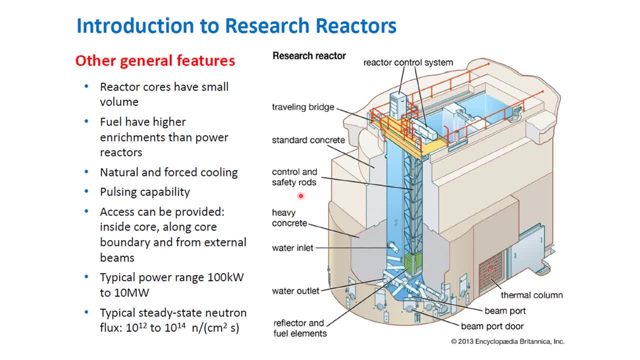 concrete for biological shielding, of course, your control and safety rugs, and then yours- uh, you have a standard concrete, and then you also have here a traveling, traveling bridge which allows for the movement of your core. you have here your thermal column and your beam port, and then your beam port door to allow access to your neutrons. so this design. 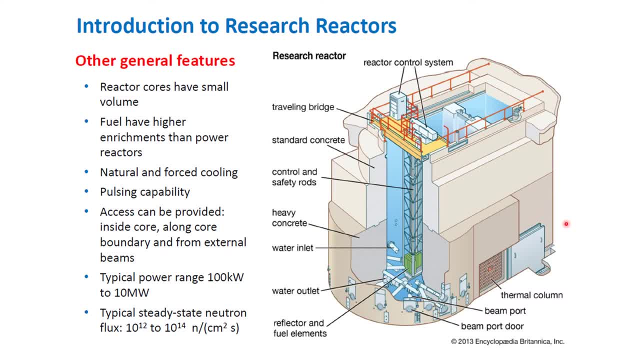 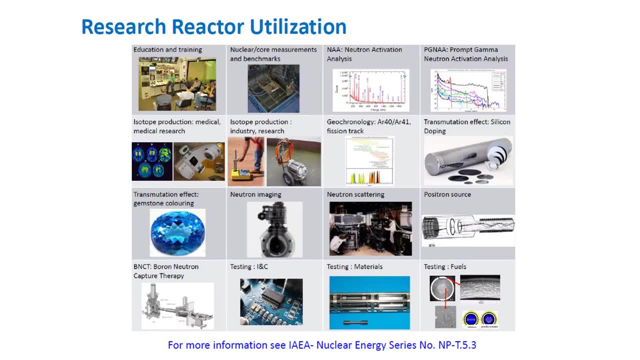 here is actually similar to the design of the philippine research reactor one in the philippine nuclear resource institute. we now cover the different applications of your research reactor and we are going to cover this one one by one. if you actually want more information about the philippine nuclear research reactor, you can go to the philippine nuclear research. 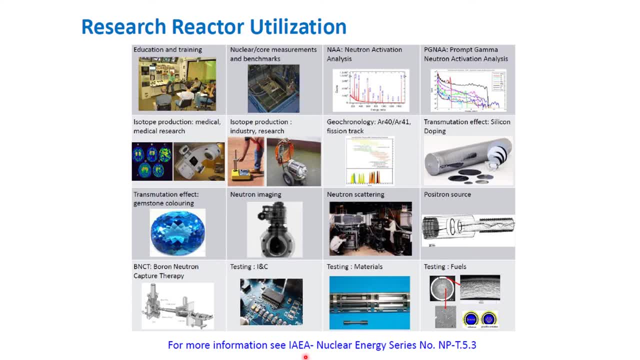 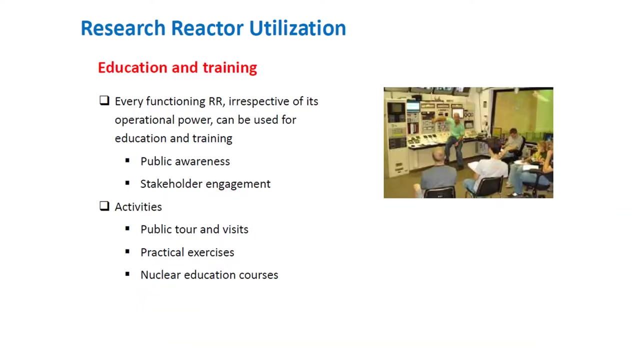 reactor website you can look up your ie iaea nuclear energy series number and np-t- that 5.3, wherein you can have more information about this research reactor utilization utilization or your research reactor applications. your research reactor can be used in education and training, wherein every functioning research 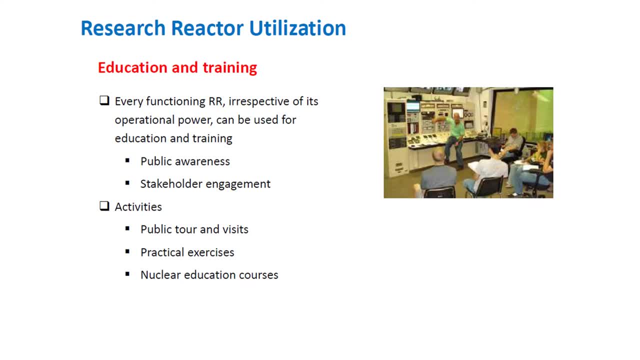 reactor facility can be used in education and training, where in every functioning research reactor facility, irrespective of its operational power, can be used for education and training when reviewing the potential uses of existing reactors, this type of application is not to be dismissed as being a trivial or unprofitable mission. on the contrary, it needs to be thoroughly explored and utilized. 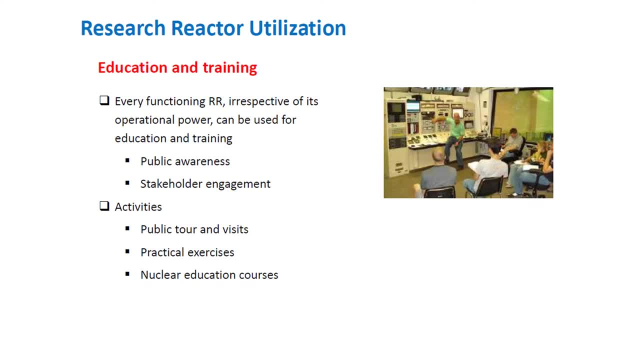 to the benefit of the facility as much as the university. faculty commitments and facility staff revenue requirements allow educating the public to be more knowledgeable of the facilities design. summers can be. Waterfront recreation is normallyoba certain reality. training programs to núcleo affairs usually results in less opposition and 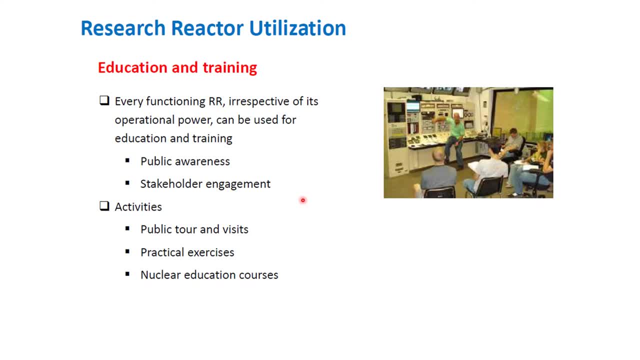 potentially more support on related issues for public awareness. similarly, educating and training civil society, from primary students and the general public through public tours and visits or public tours to university courses and power reactor operator training so we can have practical exercises and nuclear education courses related to education and training. 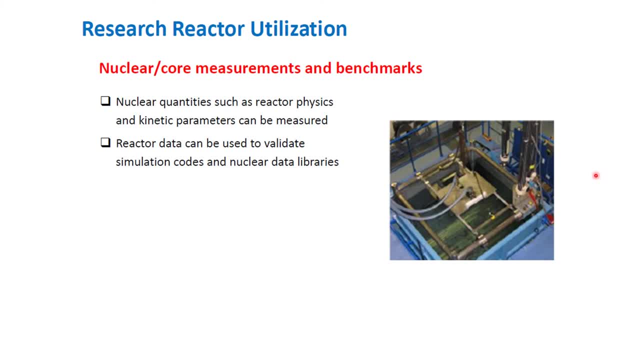 we also use your research reactor for nuclear or core measurements and benchmark we're in. nuclear quantities such as reactor physics and kinetic parameters can be measured, and also your reactor data can be used to validate simulation codes and clear data libraries. so if you have a simulation of 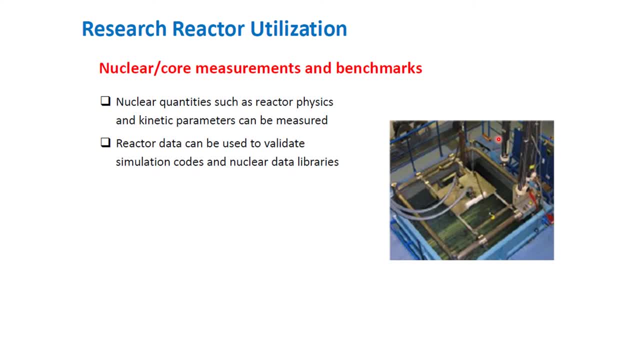 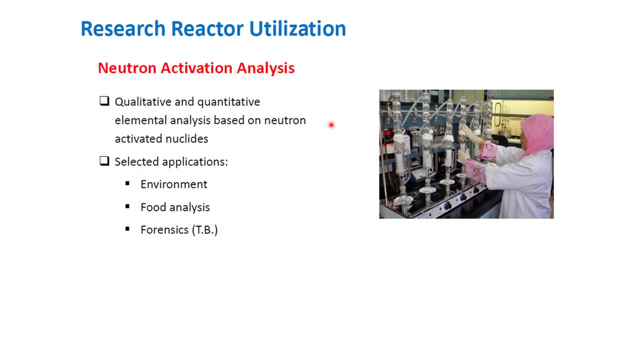 of a nuclear activity. you can use your research tracker to validate your results. your research reactor can also be used in nutrient activation analysis, or your NAA. your nutrient activation analysis is a method for the qualitative and quantitative determination of elements based on the measurement of characteristic radiation from 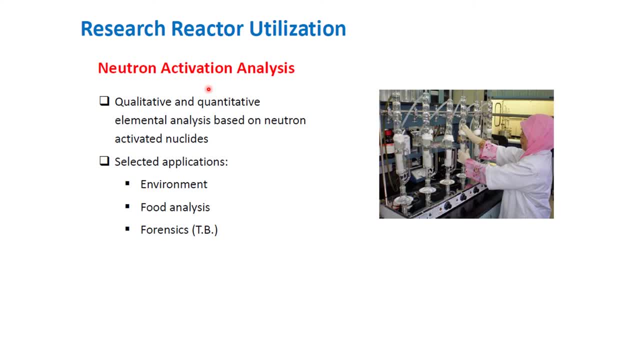 radionuclides formed directly or indirectly by neutron irrigation of the materials. the most suitable source of neutrons for size and application is usually a nuclear research reactor, and your nutrient activation analysis can be performed in a variety of ways depending on the element and the corresponding radiation. 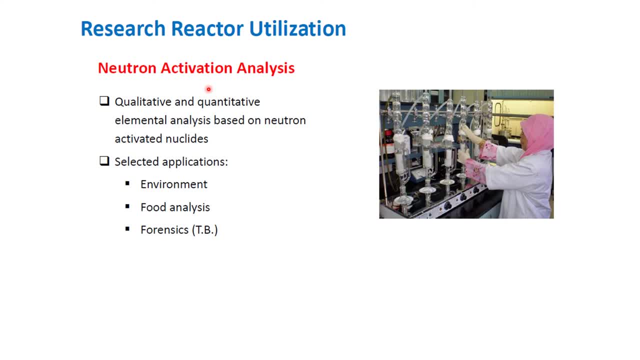 levels to be measured, as well as on the nature and extent of the difference from other elements present in the sample. next to education and training, neutron activation analysis is the most widely used application of your research reactors. almost any reactor in excess of 10 to 30 kilowatts is capable of providing a sufficient nutrient. 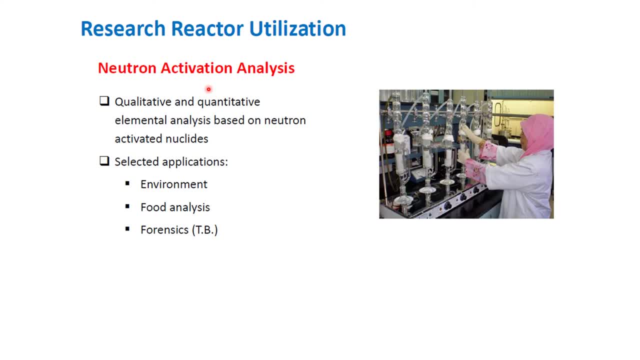 rich nutrient and nutrient efficient consuming capacity with yielding to the same level. in research, selected applications of your nutrient activation analysis is in environmental analysis, food analysis and forensics. just for example, if you know, ty cobra, which is the mentor of johannes kepler, there was actually a um issue with with his death because it was thought that he may have. 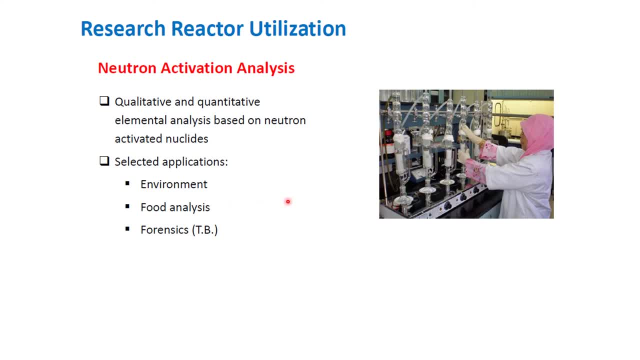 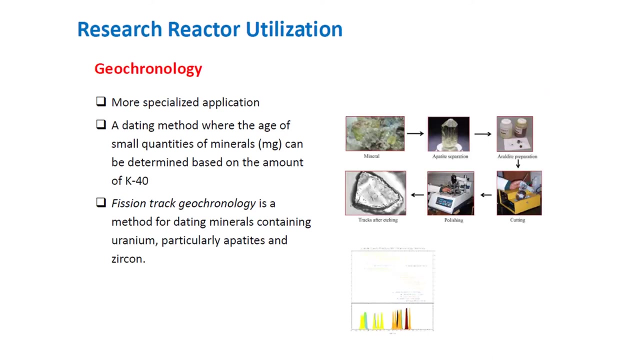 died also of poisoning, but it was done just recently by a nutrient activation analysis and was confirmed that he was actually, that he actually died of natural cause and not of of a poisoning. so that's an example application of your neutron activation analysis. the use of research reactors for geochronology is a more specialized application. 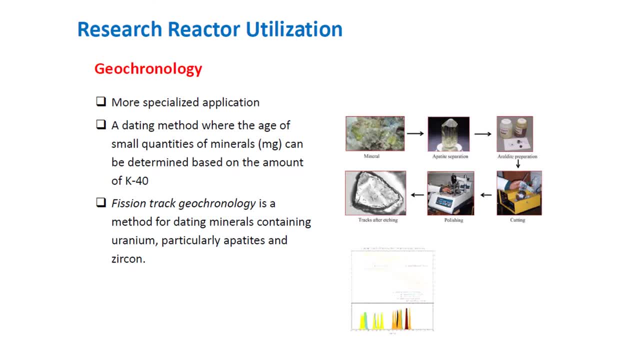 reasonable power levels are required and the user base is a relatively small but wide but widespread group of geologists from many universities and institutions. in addition, there is a tendency towards loyalty to the reactor facilities that are currently utilizing geochronological equipment, owing to the lengthy facility calibrations normally required for such equipment. a dating method where 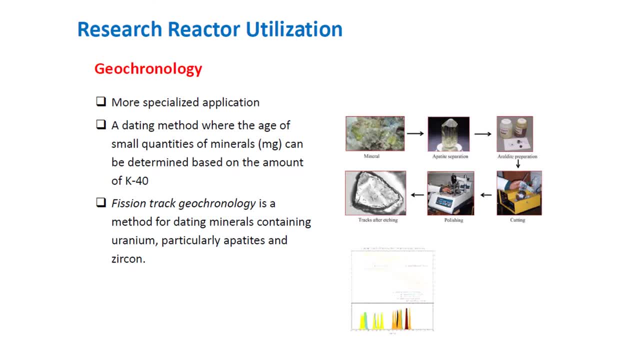 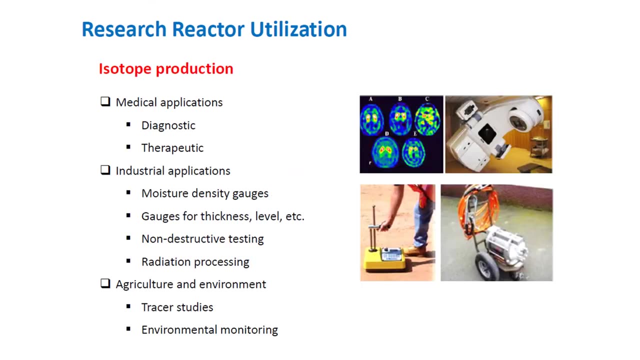 the age of small quantities of minerals. milligrams can be determined based on the amount of your weight: 40. patient trap geochronology is a method for dating minerals containing uranium, particularly hepatites and zircon. radio isotopes have a wide range of applications in various fields, including 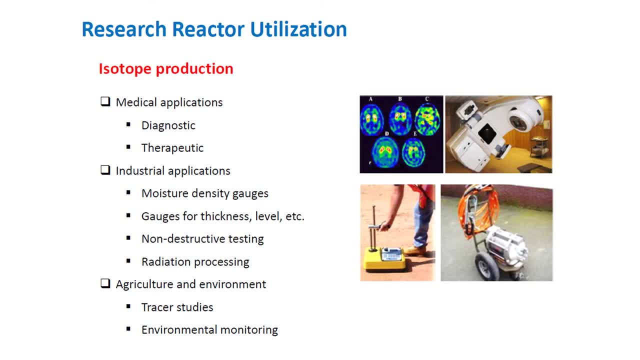 nuclear medicine industry, agriculture and research. they are produced mainly in research reactors and accelerators, involving several interrelated activities such as target fabrication, radiation of irradiated targets to processing facilities, radiochemical processing or or encapsulation in sealed sources, while the control and transportation to end users, the production of radio isotopes of 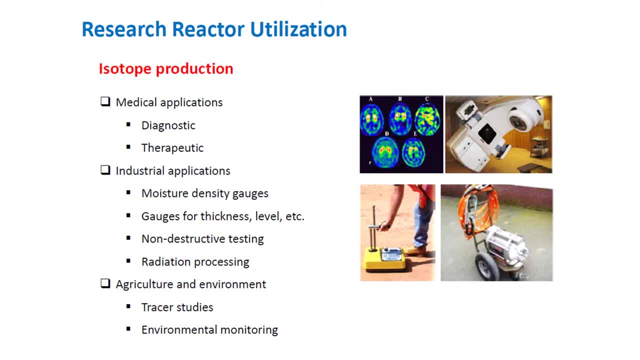 in reactors is based on neutron capture in a target material material either by activation or generation of radio isotopes from fission of the target material by bombardment with thermon neutrons, research to develop a new radio isotopes for diagnostics and therapy and in nuclear medicine, non-destructive testing and radio tracer industrial applications, as well as for 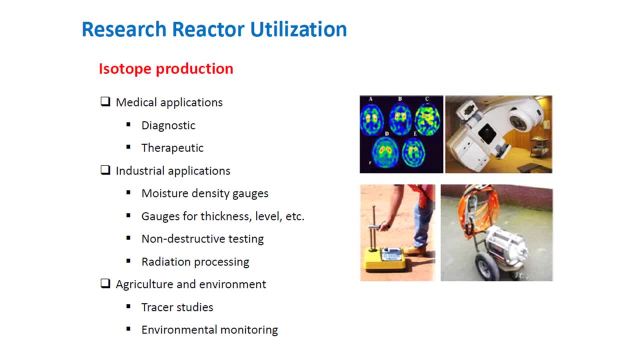 radio tracer studies in scientific research provides excellent participation opportunities for research reactors and cyclotrons for medical applications. your isotope production can be used in diagnostic and therapeutic. for industrial applications you can use it in moisture density cages, gauges for thickness level, non-destructive testing and radiation processing for the agriculture and the environment testing. you can 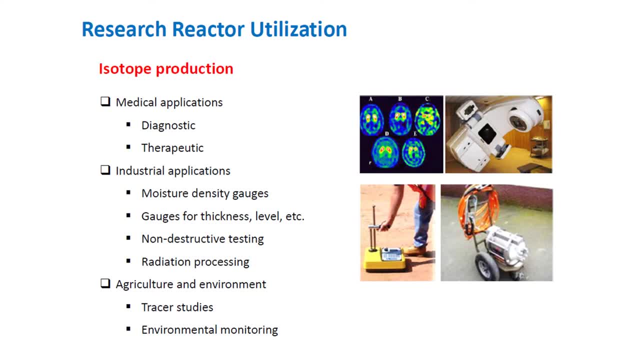 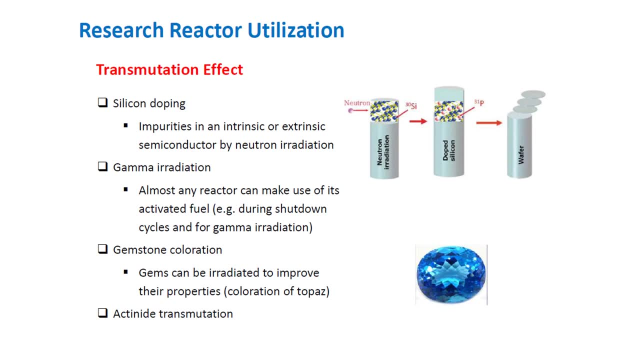 use it as tracer studies or for environmental monitoring. transmitting effects. this category includes those applications in which neutrons or gamma radiation are used to bring about a change in the material properties. the transmutation effects under discussion usually require significant fluences to induce a change in the material properties. 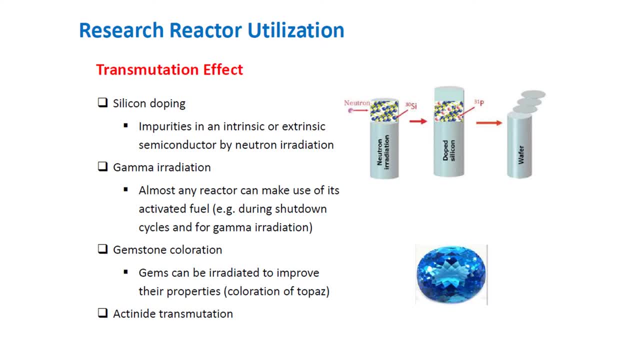 effects within a reasonable time period. this requires the application of medium and higher powered research reactors. additionally, to produce sufficient quantities of product to make it worthwhile, fairly large, uniform flux aeration positions are often required for your transmutation effect. we have your silicon doping, gamma radiation, gemstone coloration and actinide transmutation. 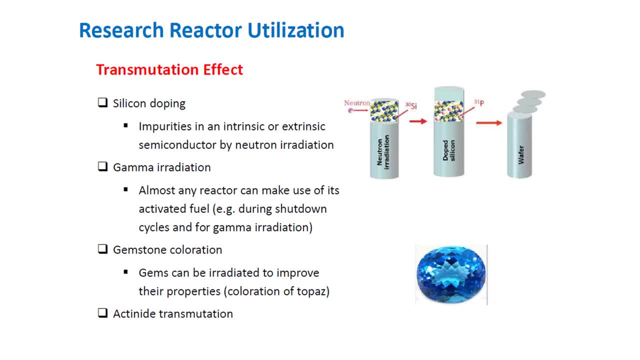 silicon transmutation doping has this process, which is called your neutron transmutation doping, doping or ntd. this is defined as the process of creating impurities in an intrinsic or extrinsic semiconductor by neutron irradiation, thereby increasing its value for various applications, the targets or candidate. 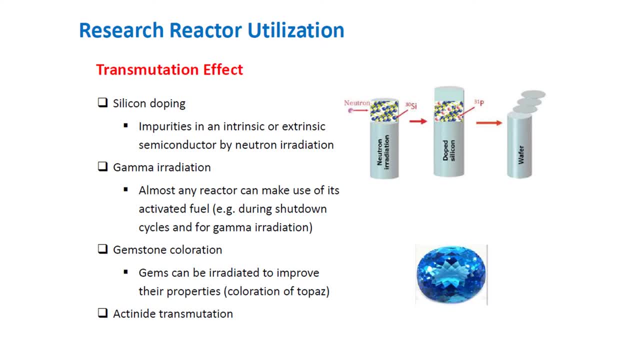 materials for ntd include gallium, arsenide, gallium, nitride, gallium, phosphide, germanium, indium, phosphide, indium selenide, mercury, cadmium, telluride and silicon, among others. of this, silicon is the currently the only target utilized for commercial neutron transmutation. 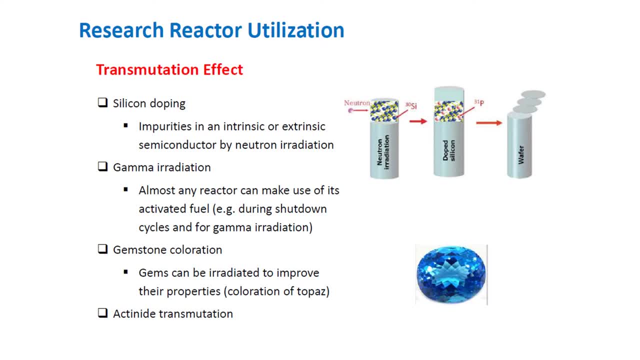 doping applications and is the most widely internationally used semiconductor material. npd technology is a preferential method for the production of extremely high silk quality silicon semiconductors due to its extremely uniform open concentration. as a result of the ability to provide excellent product quality, the demand for ntd of silicon has become an internationally 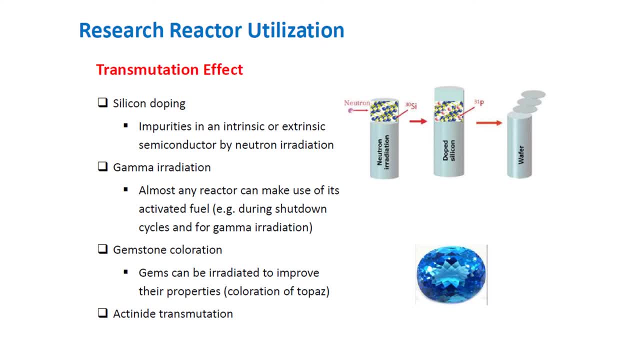 significant commercial opportunity. gamma radiation irradiation, on the other hand, can be readily developed with a relatively small investment at a research reactor, for example for irrigating plants and seeds. When assemblies are utilized, the dose rate achievable is dependent on reactor power and cooling time. Fuel element storage racks can be used to hold the assemblies during the gamma irradiation. 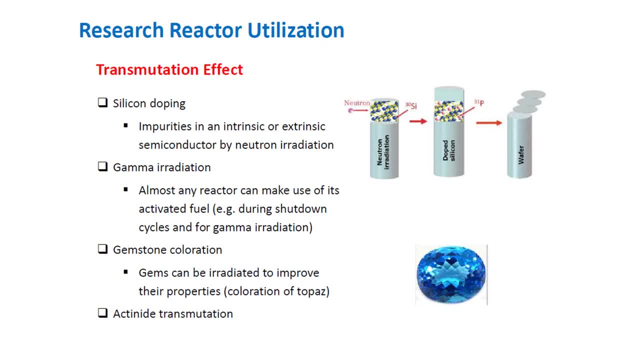 and very little extra is needed with respect to the facilities, equipment, personnel and funding. Gemstone coloration, which is an interesting application of transmutation effect, is the next thing that we are going to talk about. Gemstones may be irradiated either with neutrons or gamma-quantum high energy. 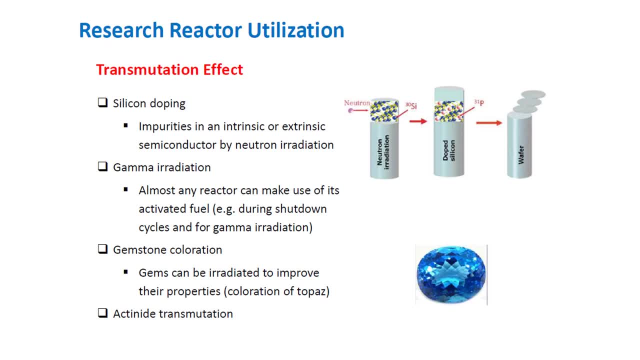 of the order of several tenths of mega-electron volt produced by electron beams to improve their properties, for example changing to a more desirable color to increase their appeal and monetary value. One of the more significant commercial neutron irradiation activities currently being performed at research reactors. 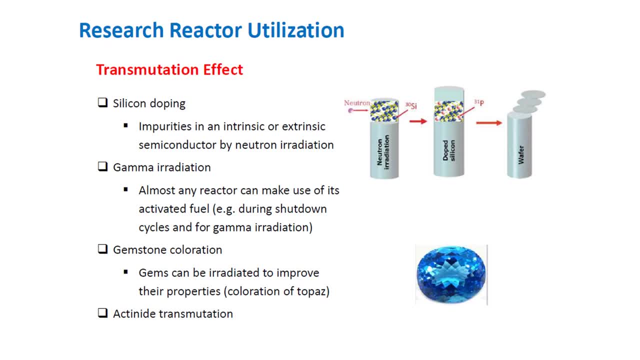 is the coloration of the gemstones. The following information is pertinent to topaz irradiation. However, before proceeding to gemstone coloration, the legality of this activity must be verified with national authorities, as several states have banned the practice, Similar to NPD, of silicon. there is a potential for the generation of a significant income through gemstone irradiation. 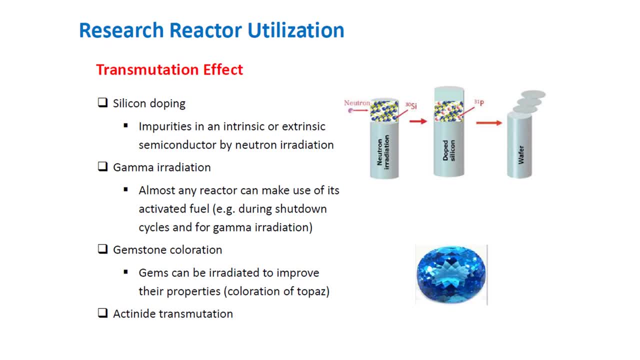 Unfortunately, due to the commercial sensitivity, there is an understandable reluctance among those performing their irradiation to disclose the specific details of their processes, in particular, for both NPD and gemstone applications. In addition, there are some difficulties associated with gemstone coloration activities that need to be avoided. 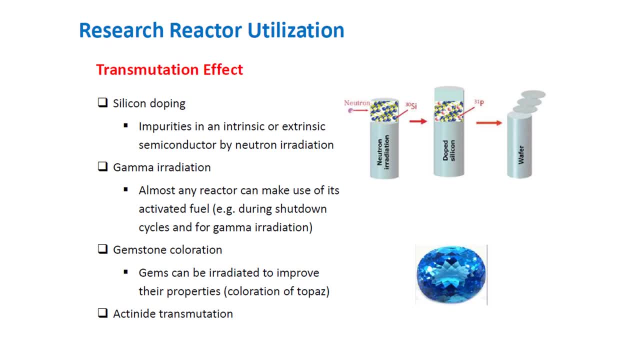 For aptinite transmutation. it has been recognized for many years that it is theoretically possible to transmute some long-lived actinides and spent nuclear fuel into shorter-lived products, thereby reducing the potential waste disposal hazard. To this end, some actinide burners have been designed, but none has yet been built for this specific purpose. 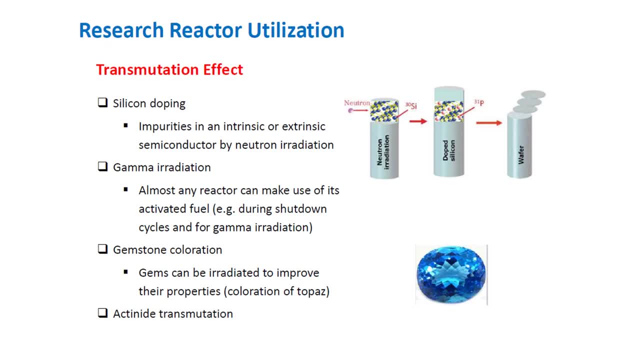 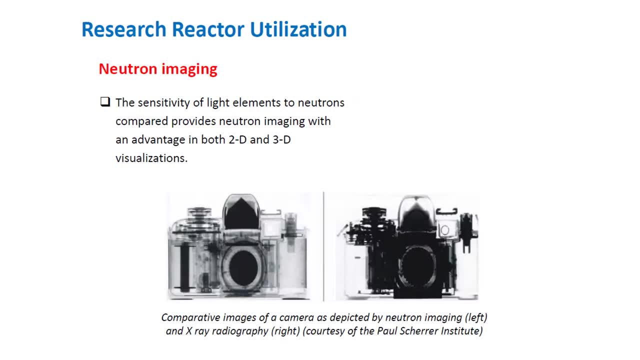 It is possible that some reactors may be utilized in the future for test irradiation of fuel plates or elements. The sensitivity of light elements to the absorption of neutrons compared with X-ray imaging provides neutron imaging with an advantage in both 2D and 3D visualizations. 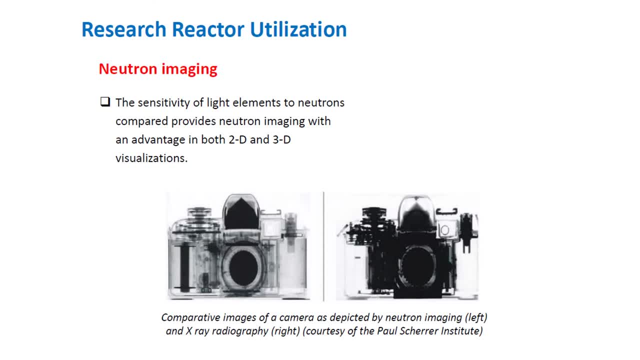 Until the 1990s, the dominant detection systems for neutron imaging were film-based. that is, you have X-ray film and converters with track-etch foils and known simply as neutron radiography. Since then, detection methods have been improved drastically. 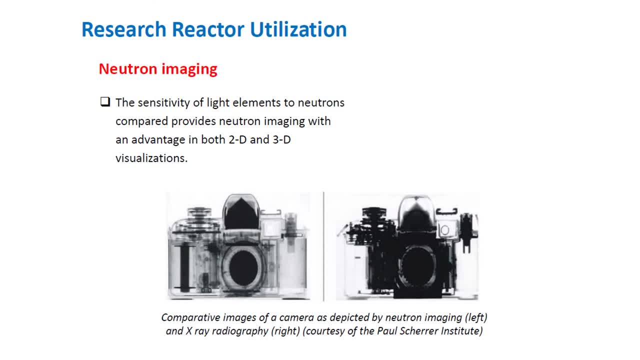 digital processing systems have been introduced and imaging beamlines have been built with the capability to scan in energy through the range in which structural materials show broad diffraction edges. In this figure here you can compare the image form by neutron imaging and X-ray radiography. 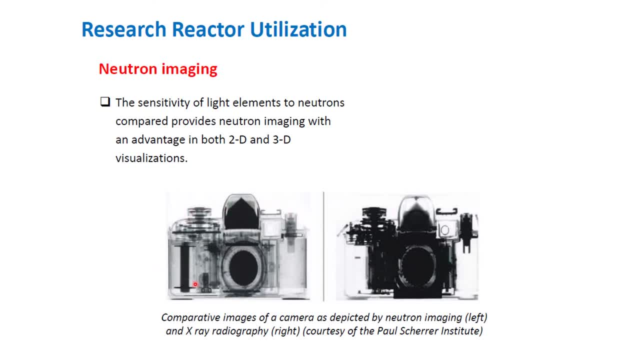 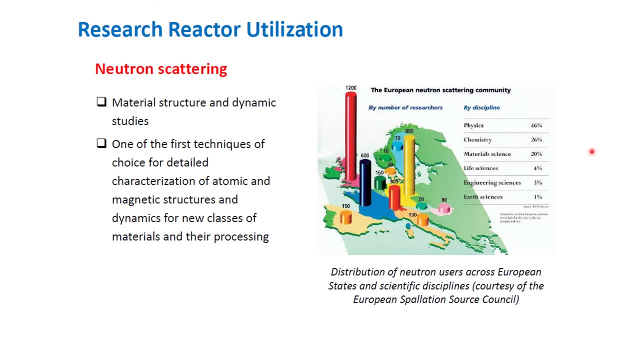 As you can see, we can see more components inside your camera with neutron imaging than your X-ray radiography. Two interactions of neutrons with matter make neutron scattering a unique probe for materials research, namely short-range strong nuclear interactions and electromagnetic interactions. 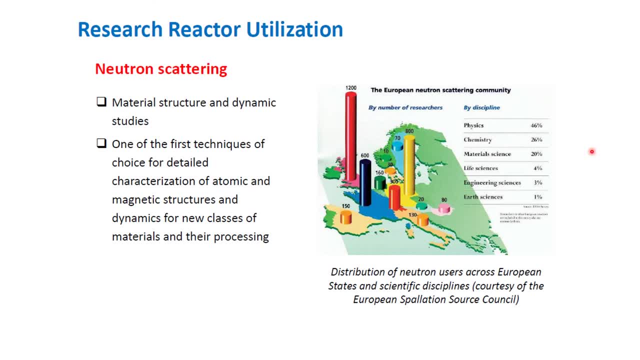 due to the net energy of the neutron Neutronic magnetic moment In particular. as neutrons have no net electric charge, they can penetrate the bulk of materials, making metallic objects largely transparent to their transmission. Furthermore, thermal neutrons play a crucial role among many other engineering functions. 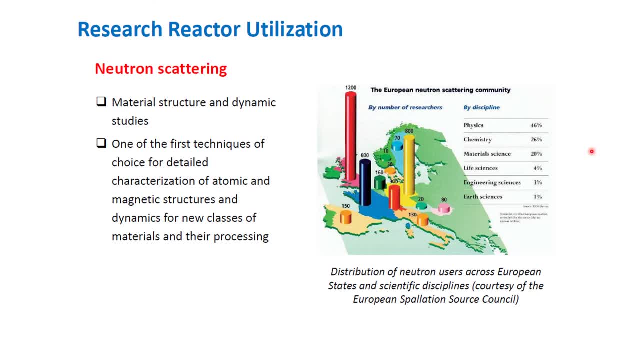 In locating light atoms such as hydrogen and oxygen in intricate structures. they can be used to solve the arrangement of magnetic moments in complex magnetic systems and accessing residual stress distribution in mechanical components. Typical example media include hydrogen storage materials, electrolyzed and battery materials and magnetic films. 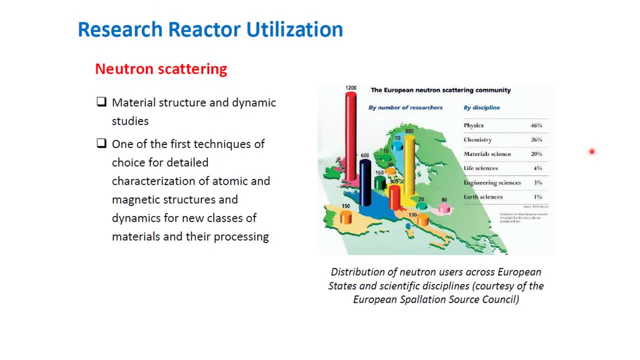 Exotopic substitution is exploited to elucidate the precise location of hydrogen atoms, for example, in polymers and biological molecules. Material structure and dynamic studies is what is usually used in your neutron imaging, And this is one of the first techniques of choice for detailed characterization of atomic and magnetic structures. 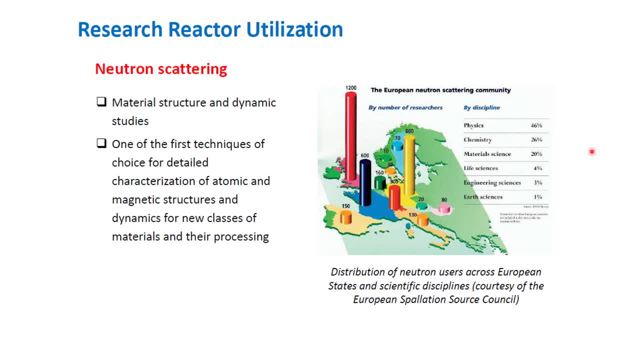 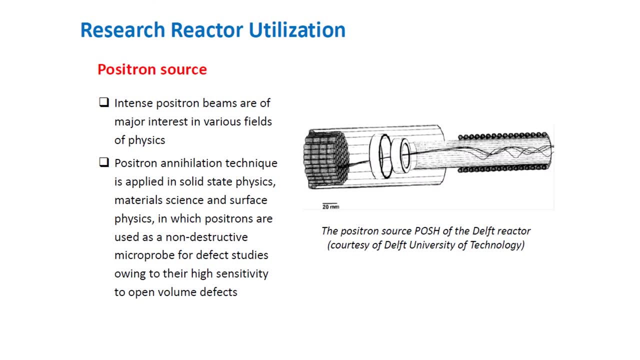 and dynamics for new classes of materials and their processing. High intense positron beams are of major interest in various fields. High intense positron beams are of major interest in various fields. The positron annihilation technique is applied in solid-state physics, material science and surface physics. 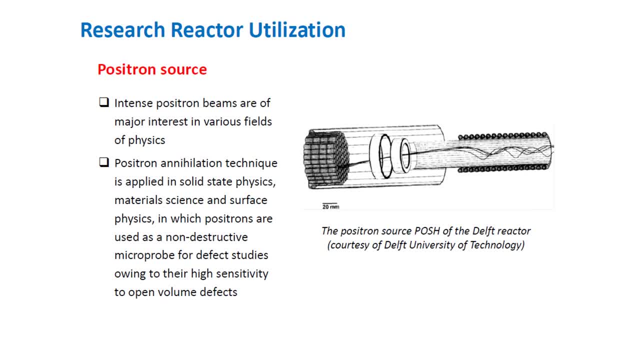 in which positrons are used as non-destructive microprobe or defect studies, owing for their high sensitivity to open-volume defects In atomic and nuclear physics, scattering experiments with positron and positronium, as well as the investigation of positronium and its excited states. 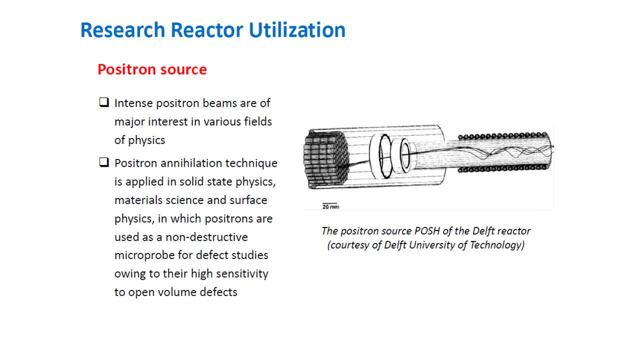 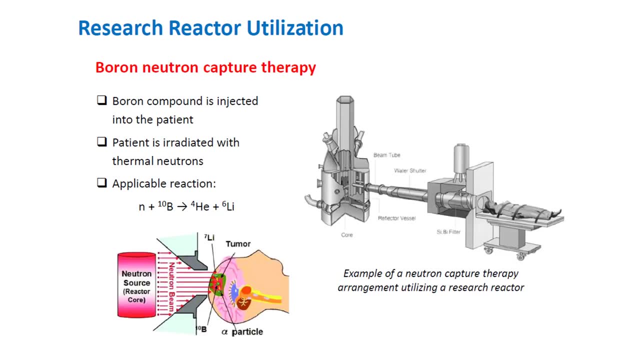 require intense positron beams. When boron-10 absorbs a neutron, it emits an alpha particle which is highly ionizing and has a range in tissue about equal to the diameter of a cell. The reaction is you have a neutron absorbed by boron-10, produces an alpha particle and lithium-6. 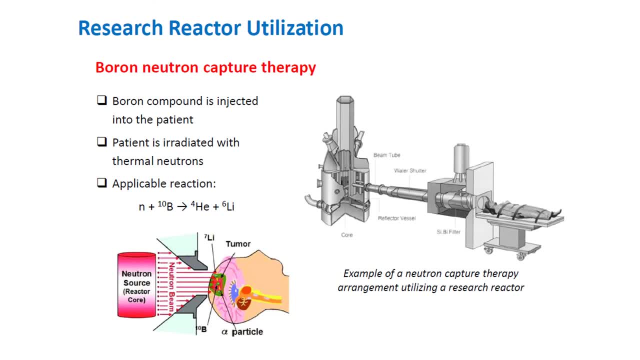 The applicable methodology in boron-neutron carbon therapy, or BNCT, is thus to inject a tumor with a borated compound that irradiates it with thermal neutrons. If the conditions are right, the tumor dose is much higher than that of the rest of the surrounding tissue. 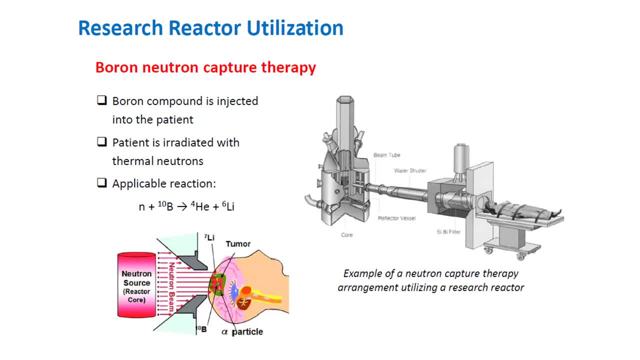 resulting in the preferential eradication of the tumor cells. Thermal neutrons are desired at the tumor location because the boron-10 interaction probability is much higher with slower neutrons. Surface or shallow tumors can therefore be irradiated with thermal neutrons. 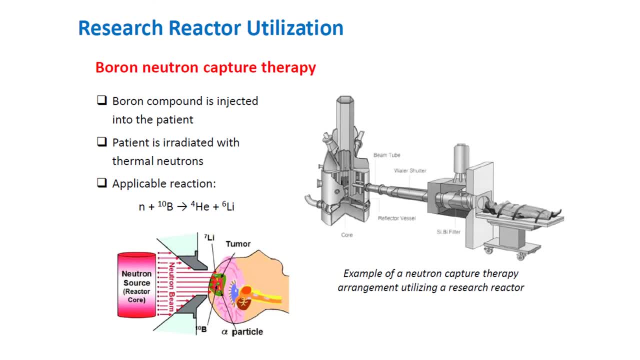 while those at a depth of a few centimeters can be irradiated with epithermal neutrons, which are then thermalized as they pass through and interact with the overlying tissue. Thermal neutrons are also useful for BNCT research involving cell cultures or small animal irradiations. 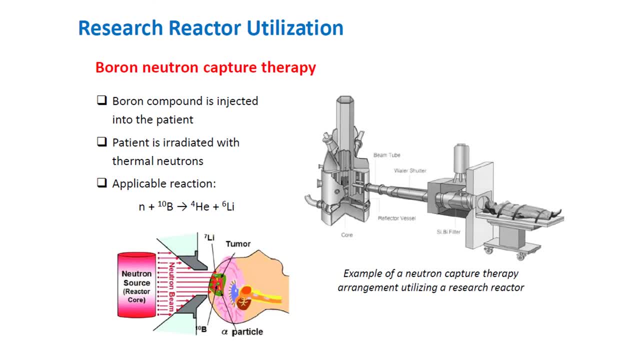 Although most of the neutron capture therapy currently practiced makes use of boron compounds, other compounds such as gadolinium can also be used. The majority of neutron capture therapy research is focused on malignant melanomas and brain tumors, particularly glioblastoma multiforme. 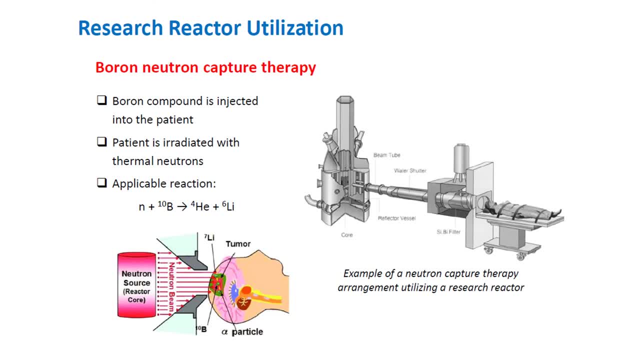 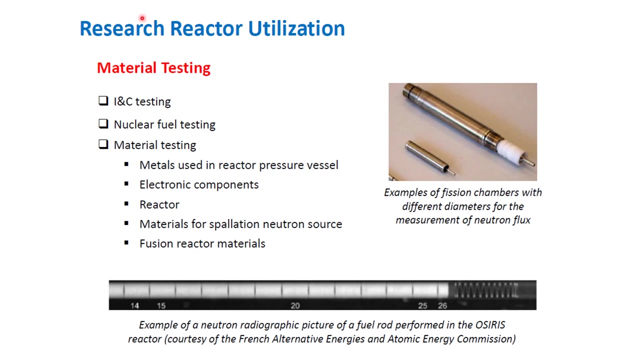 Current research efforts are directed towards providing the dose to the tumor in a short period of minutes instead of hours and reducing the dose to normal tissue through higher flux, Better neutron energy selectors, shielding and columnation, and better drugs. One of the major applications of research reactors, whether low, medium or high power. 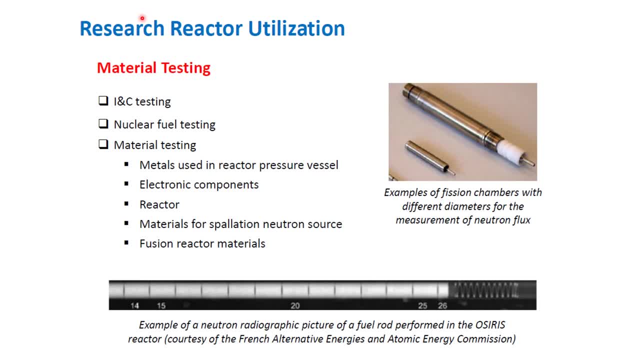 is the ability to be utilized to perform testing and calibration experiments. This can be applied to various types of instrumentation, as well as to materials intended for use in either nuclear fuels or reactor structural components. Some aspects of such applications include IC testing, nuclear fuel testing and material testing. 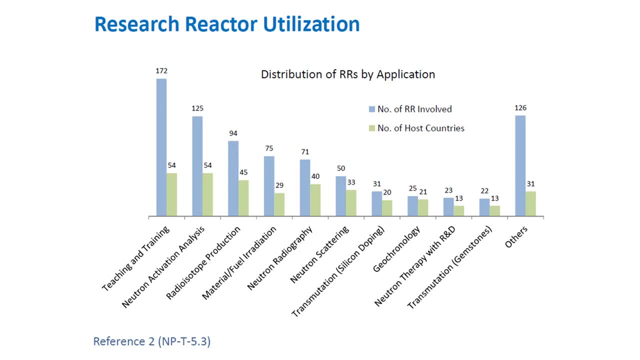 These are the distribution of your research reactors by applications. The blue bar is for the number of research reactors involved and the green bar is for the number of host countries. As you can see, teaching and training is at the top, with 172 research reactors involved. 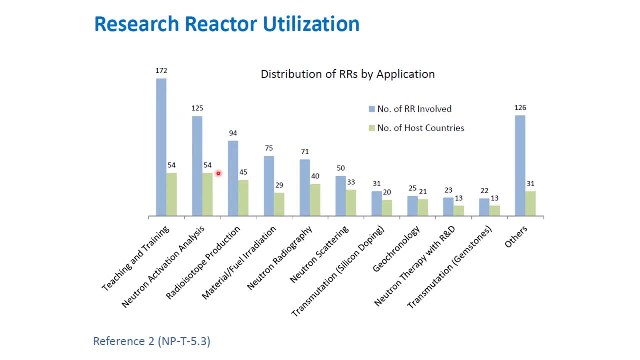 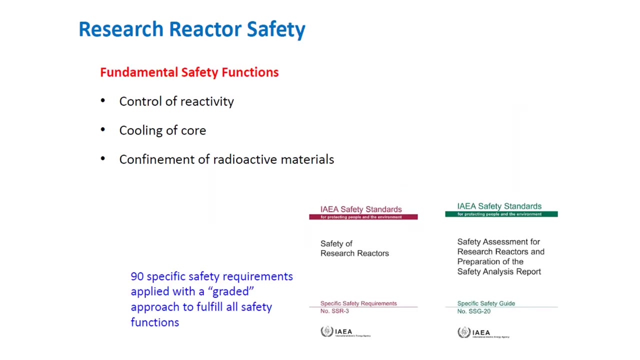 This is followed by your neutron activation analysis and radioisotope production. Other applications are also at the top of the list, which are not discussed here. It is also important to talk about the research reactor safety, and these are the fundamental safety functions that need to be addressed. 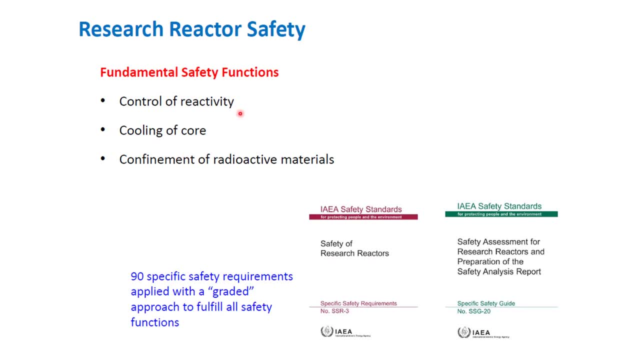 You have your control of reactivity or neutron population, the cooling of the core and confinement of radioactive materials. The following IAEA safety standards can be used as guidelines for the safety of research reactors and another one is also for the safety assessment for research reactors. 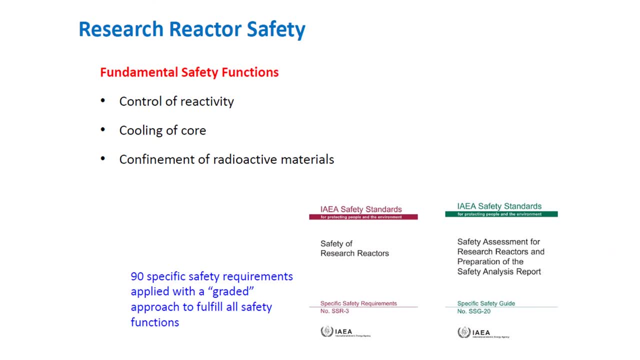 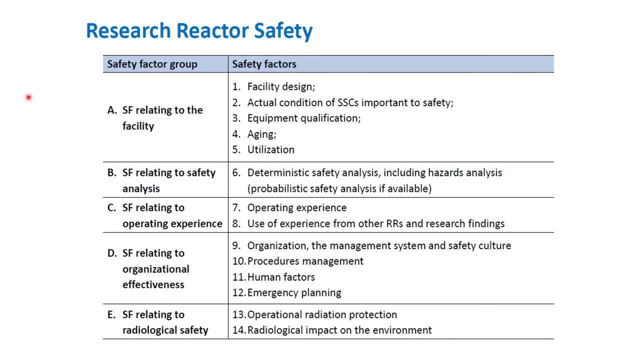 and preparation of the safety analysis report. The safety factors is actually a comprehensive list which includes facility design, actual condition of SSCs important to safety equipment qualification, aging, utilization, deterministic safety analysis, including hazard analysis, operating experience, use of experience from other research reactors and research findings. 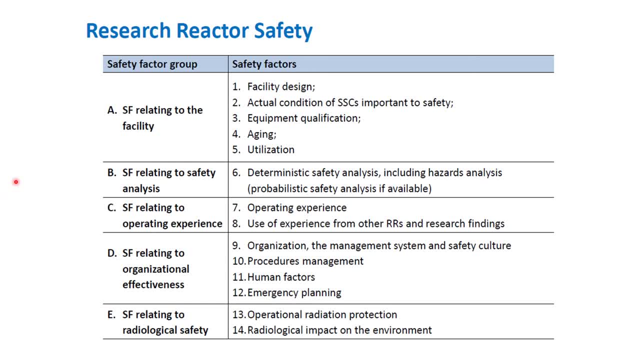 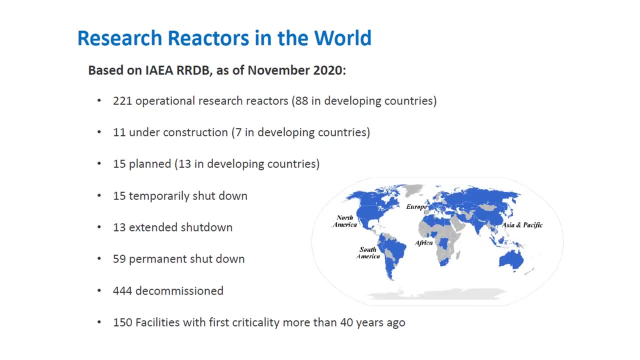 organization, the management system and safety, culture, procedures, management, human factors, emergency planning, operational radiation protection and radiologic impact duty environment. Based on IAEA, as of November 2020, we have done 221 operational research reactors, wherein we have 88 in developing countries. 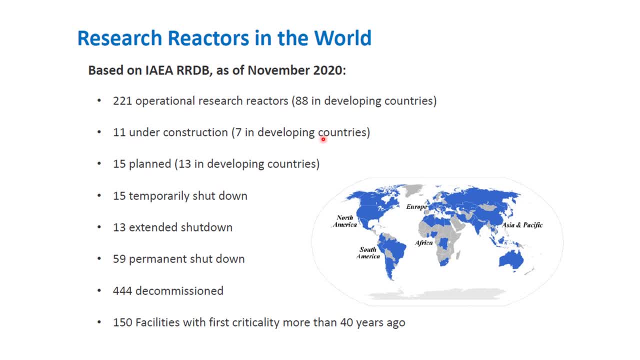 11 are under construction, 7 are in developing countries, 15 planned, 13 of which are are from developing countries, 15 temporarily shutdown- including here is your PRR1, and 13 are in extended shutdown. 59 are in permanent shutdown. 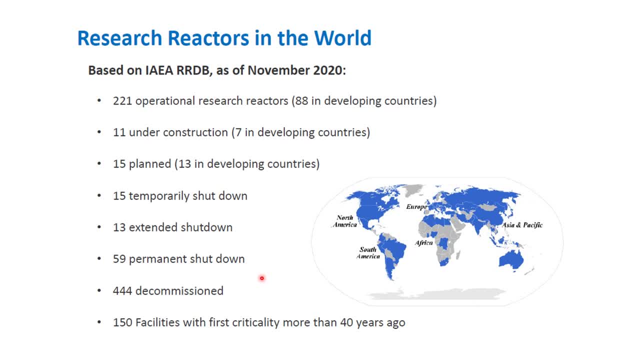 and 444 are in decommission: 150 facilities with first criticality more than 40 years ago. As you can see here, many of the research reactors are in decommission, with a number of up to 444.. And this is because. 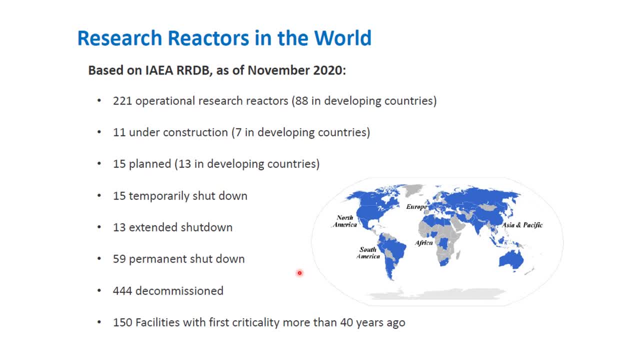 when your research reactor already fulfilled or already finished the project or has already finished the research going on, it can already be directly decommissioned. And also, research reactors are more easily be decommissioned as compared to your power reactors. So this is the same data. 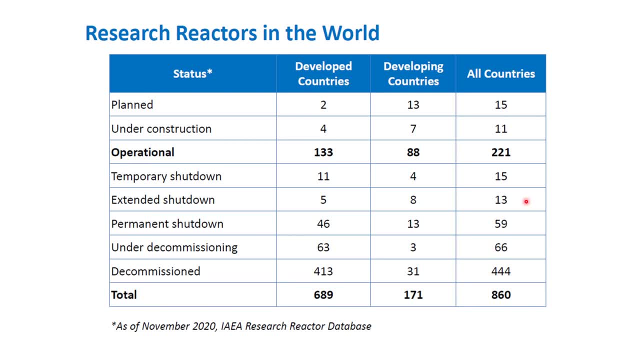 for your research. reactors in the world, just in table form. So totally we have 133 operational in developed countries and 88 in developing countries. 413 are decommissioned in developed countries and 31 are decommissioned in developing countries. 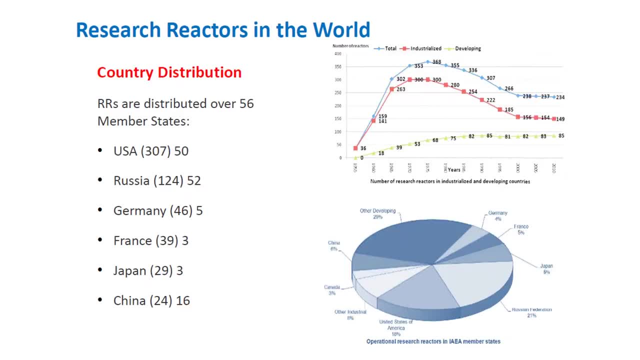 In terms of country distribution. as you can see, most of the research reactors that are operating are found in industrialized countries, But there is also an increasing trend for research reactors in developing countries. Research reactors are distributed over 56 member states, and most of the research reactors are concentrated in. 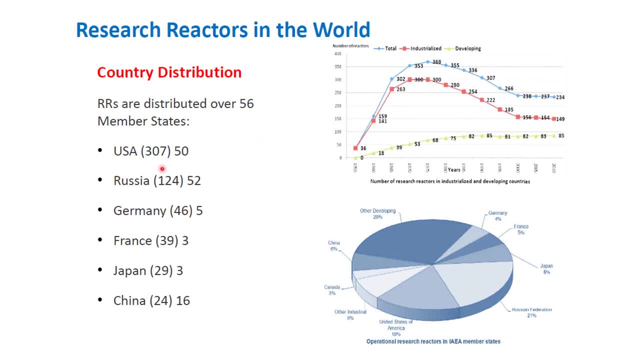 the USA with 307 and 50 plants, Russia with 124, 52 plants, Germany with 4 to 6, 5 plants, France with 39, and 3 plants And Japan 29, 3 plants. 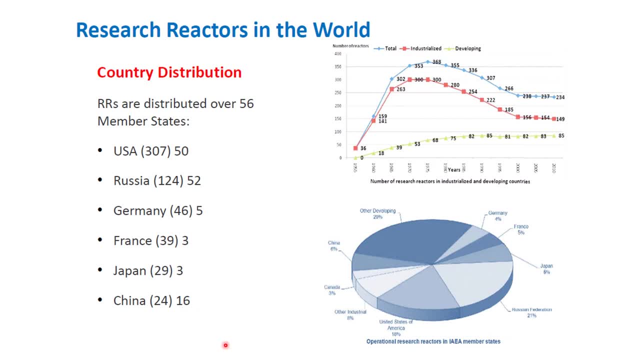 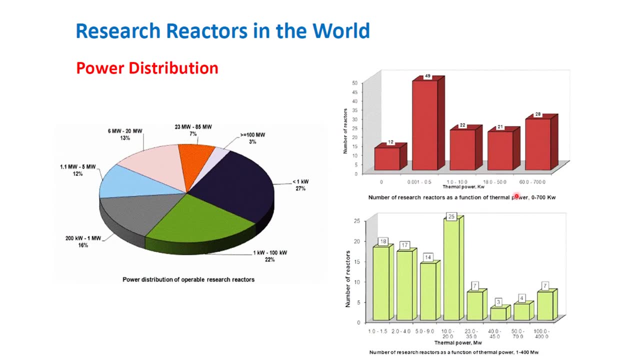 And lastly, you have China with 24 and 16 plants. This is the power distribution of the research reactors in the world. So most reactors have greater than 1 kilowatt of around 27%, And we have research reactors. 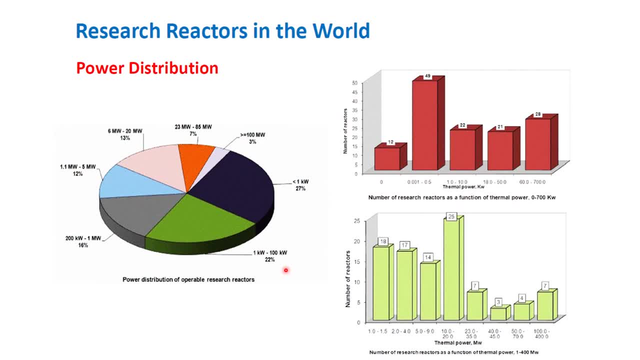 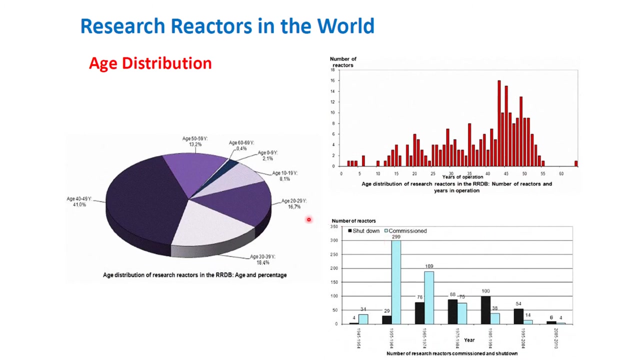 that power distribution from 1 kilowatt to 100 kilowatts And the smallest one is a research reactor with less than or equal to 100 megawatts of power, which is only around 3%. For the age distribution, many of our research reactors of around 41%. 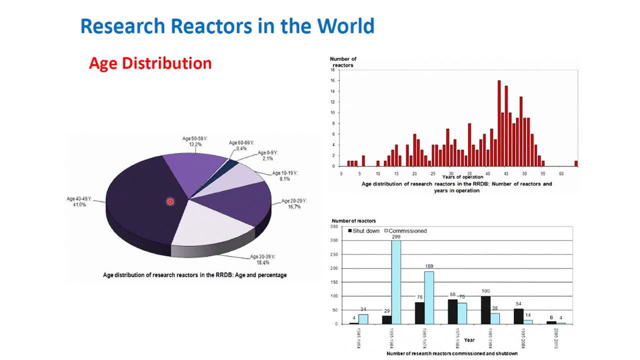 have age 40 to 49 years, And it's followed by research reactors aging 30 to 39.. And you have your research reactors aging 20 to 29, with 16%, And it's followed by research reactors aging 50 to 59 years old. 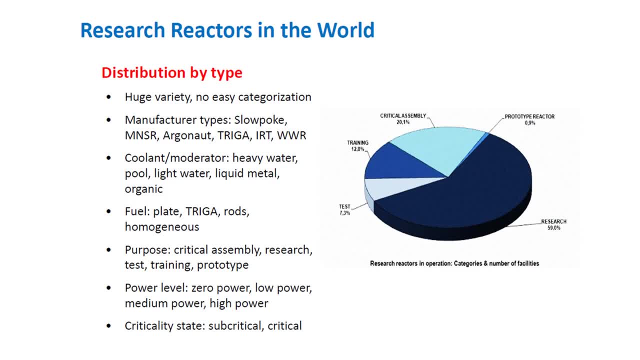 For the distribution by type. unlike your power reactors, wherein we can easily group your reactors by type, your research reactors have huge variety and there's no easy categorization. For example, we can group them by manufacturer types. You have your SLOPO. 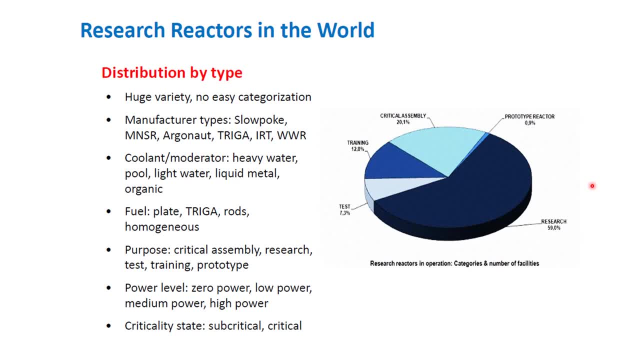 MNSR, Argonaut, Triga, IRT, UR. We can also group them by coolant or moderator. You have your heavy water, pool, light water, liquid, metal and organic. We can also group them in terms of UL type. 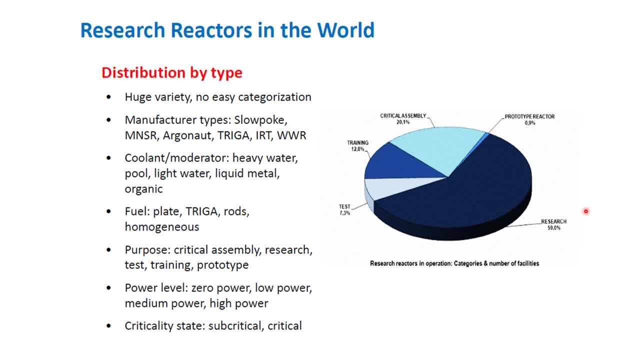 the plate, Triga rods and homogeneous. And, of course, for the purpose, we can group them by critical assembly, research, test, training or prototype. We can also group them in terms of power level: zero power, low power. 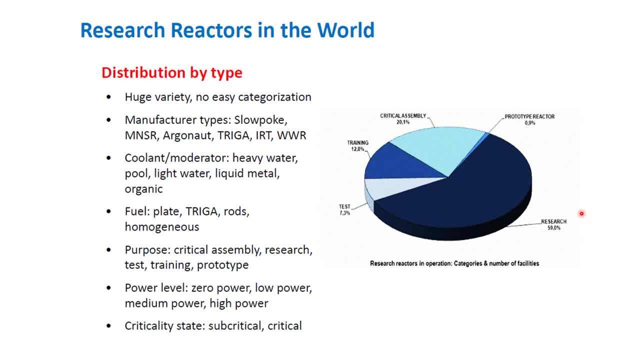 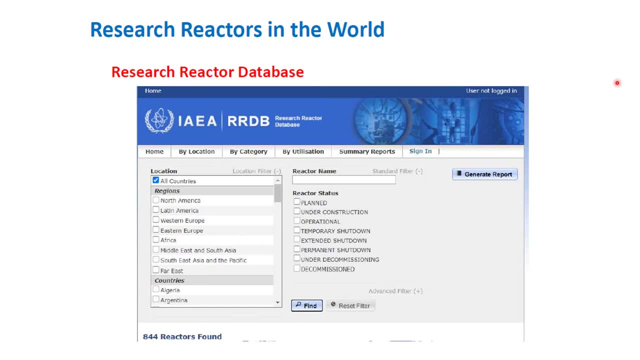 and high power And the criticality state. you can group them into sub-critical or critical. This is the research reactor database of the IADA, which you can view later. This is constantly updated for you to view research reactor statuses in different regions and in different countries. 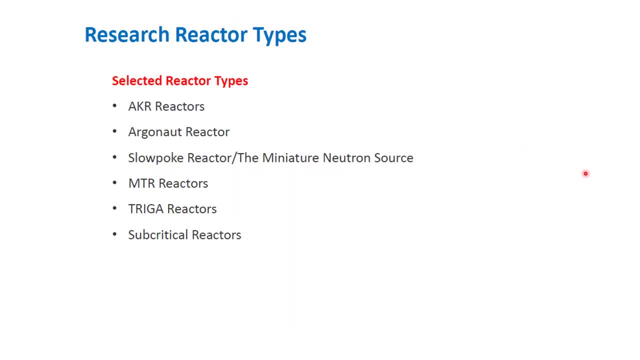 Now let's discuss some selected reactor power types. You have your AKR reactors, argonaut reactors, slowpoke reactor or the miniature neutron source, your MTR reactors, Triga reactors and sub-critical reactors. The AKR reactor is from the German. 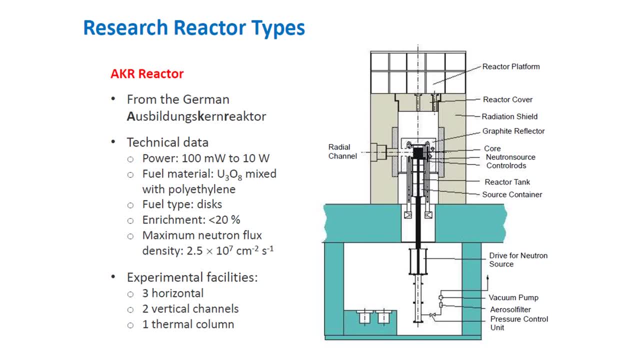 Ausbildung Kern Reaktor which directly translates to neutron training reactor. Some technical data about AKR reactors: The power is around 100 megawatts to 10 watts. The fuel material is U3O8 mixed with polyethylene And enrichment is less than 20%. 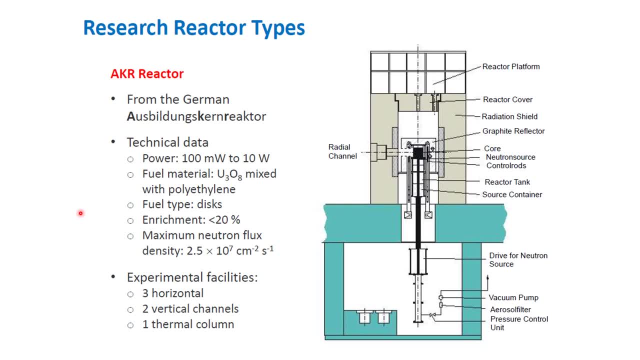 with maximum nutrient flux density of 2.5 times 10 to the 7.. It has the following experimental facilities: three horizontal, two vertical channels and one thermal column. So it basically contains the same, or the basic components of a research reactor. 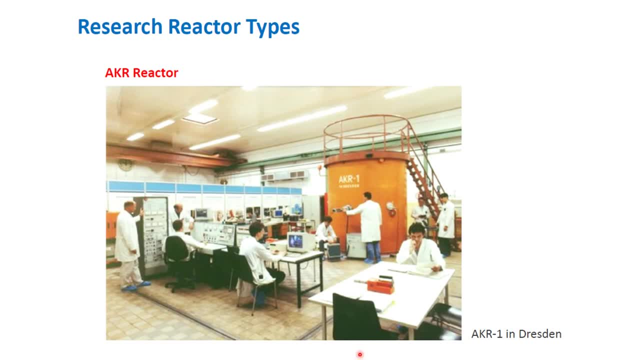 This one here is an image of the AKR-1 reactor in Dresden. This one here, this barrel here, contains your AKR reactor And around it are your nuclear scientists And, as you can see, the scientists are working close to your reactor. 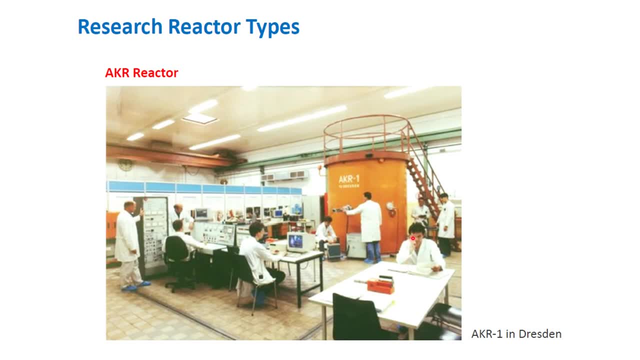 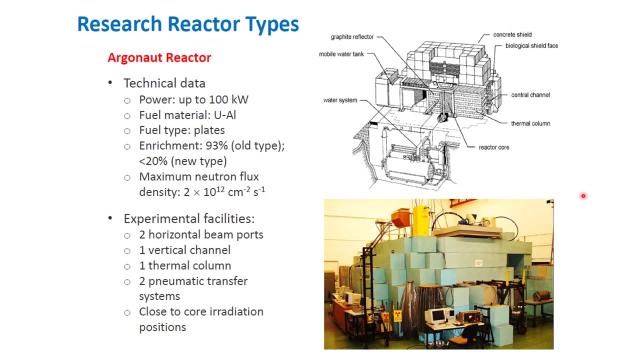 which tells us that the post-threat of radiation by the AKR reactor is very small. The next type of research reactor that we're going to talk about is the Argonaut reactor, which contains the following technical data: A power up to 100 kilowatts. 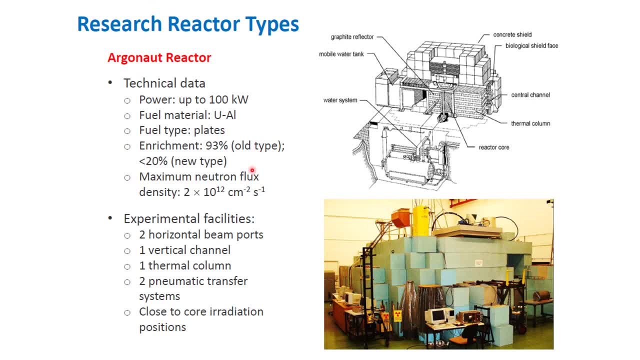 The fuel is uranium, aluminum, And the enrichment is 93% for the old type and less than 23% for the new type. Some experimental facilities include two horizontal beam ports, one vertical channel, one thermal column, two pneumatic transfer system. 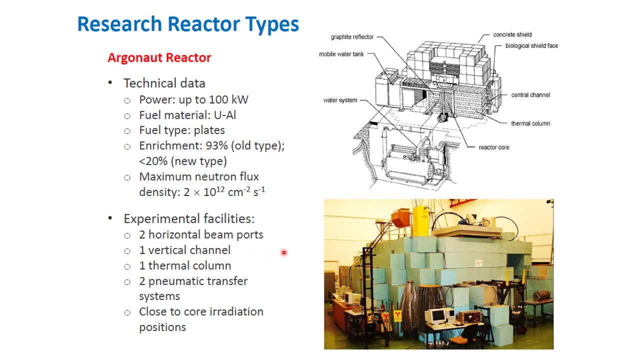 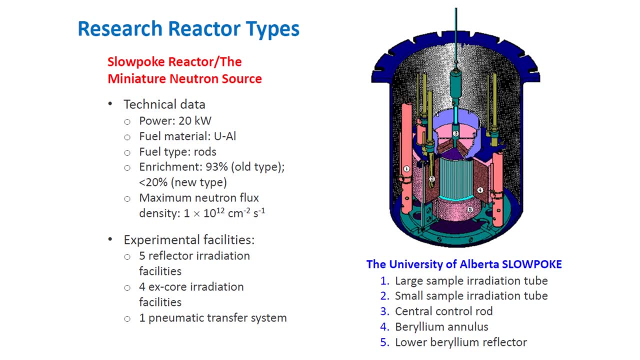 and close to core radiation positions. Next we have your slowpoke reactor or the miniature neutron source. The power can be produced is up to, or power used is, 20 kilowatts. Fuel type is uranium. aluminum Fuel type is uranium. 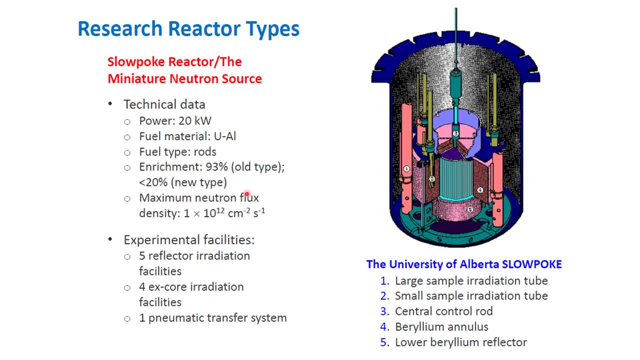 Fuel type is rods And this argin enrichment 93% for old type and 20% less than 20% for the new type. It contains five reflector irritation facilities, four X-core irritation facilities and one pneumatic transfer system. 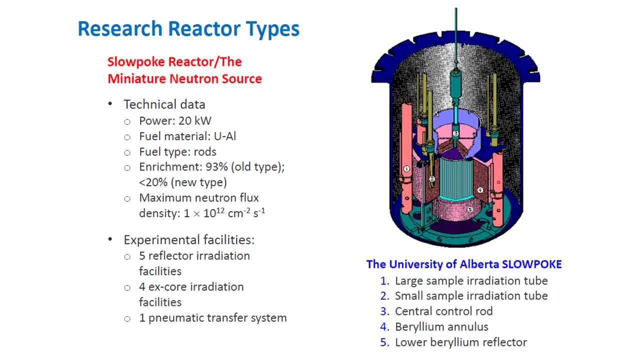 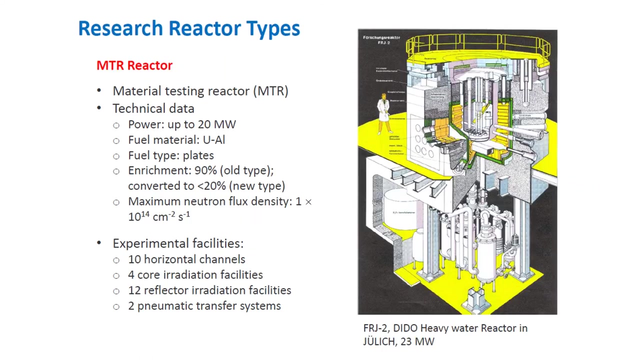 And this is the schematic diagram of the slowpoke at the University of Alberta And, as you will see, many of the universities now has research reactors, because these research reactors are used in educating new breeds of reactor scientists and also for research. Then we have the MTR reactor. 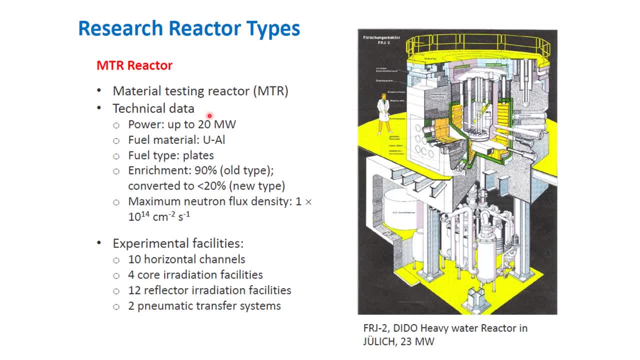 which is a material testing reactor. Some technical data: We have a power up to 20 megawatts, Fuel type is uranium, aluminum. Fuel type is plates, And then it contains 10 horizontal channels, 4x4 irradiation facilities. 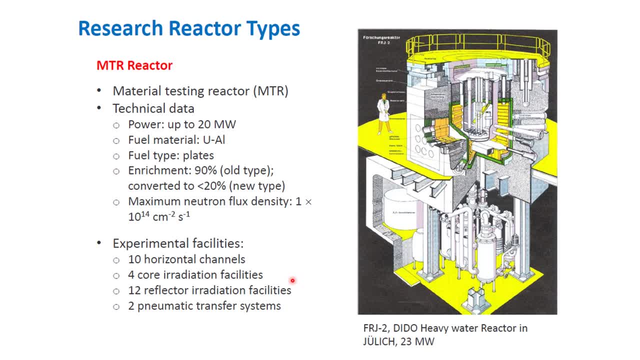 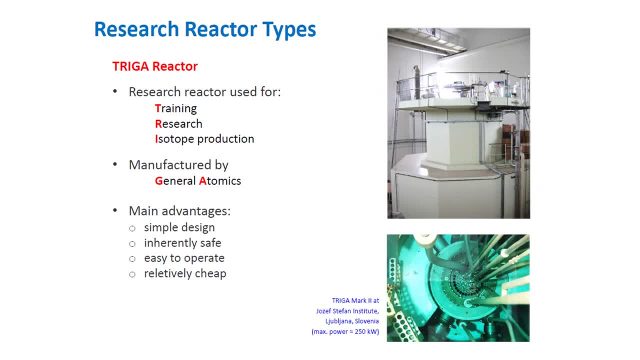 12 reflector irradiation facilities and 2 pneumatic transfer systems. So your material testing reactor, MTR. Then we have your TRIGA reactor. TRIGA basically stands for Training, Research, Isotoproduction and General Atomics. 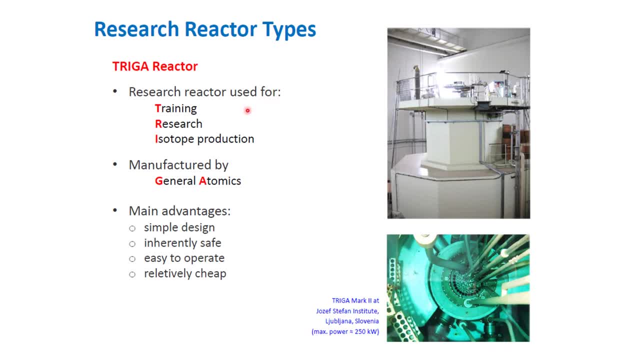 So the acronym. the acronym stands for the research reactor, where the research reactor is used for, and its manufacturer. manufacturer, the General Atomics. It has main advantages: that it is simple in design, inherently safe, easy to operate and relatively cheap. 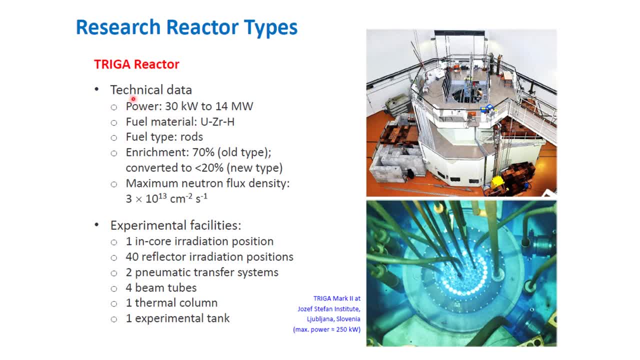 Some technical data for your TRIGA reactor. The power is 30 kilowatts to 14 megawatts. Fuel type is uranium, draconium and hydrogen. Fuel type is rods. Enrichment is 70% for the old type. 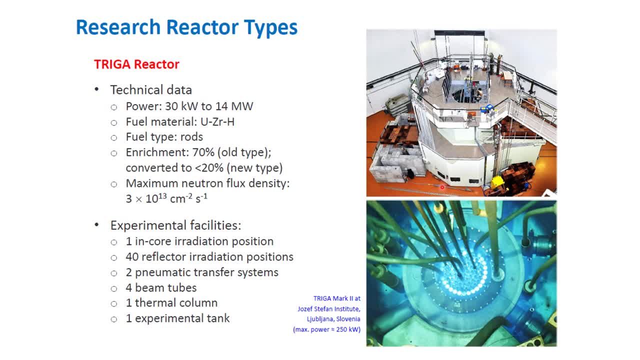 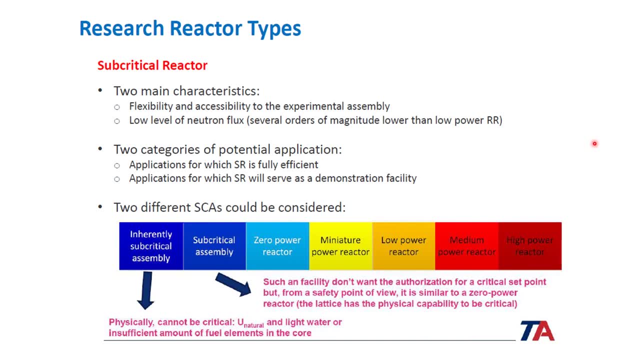 and less than 20% for the new type. And the last that we're going to talk about are your subcritical reactors. We're going to talk, we're going to emphasize, your subcritical reactors, as this is the type of reactor that we are building. 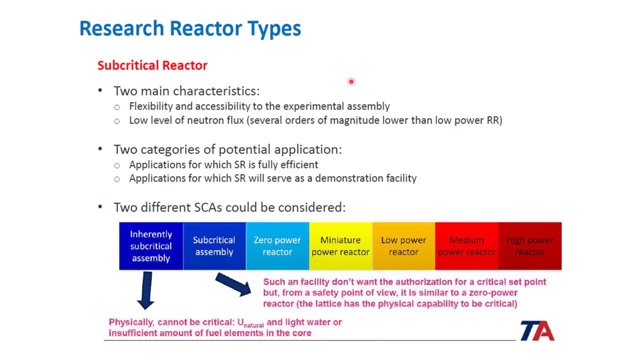 in the Philippine Nuclear Research Institute. It has two main characteristics: flexibility and accessibility to the experimental assembly and low level of different flux of several orders of magnitude lower than low power research reactors. It has two categories of potential application: One application for your subcritical reactor. 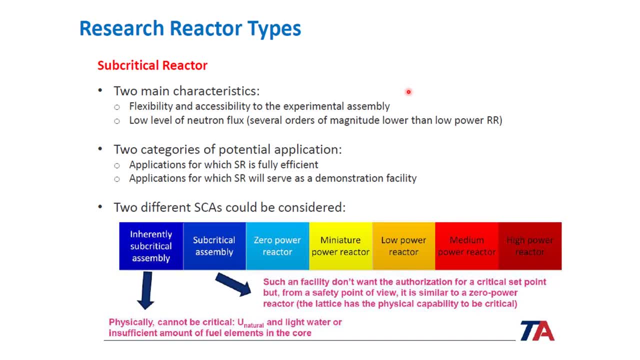 is fully efficient and applications for which your subcritical reactor will serve as a demonstration facility. And we have two different SCAs that could be considered. First is the inherent subcritical assembly. So SCAs stand for your subcritical assembly Physically cannot be critical. 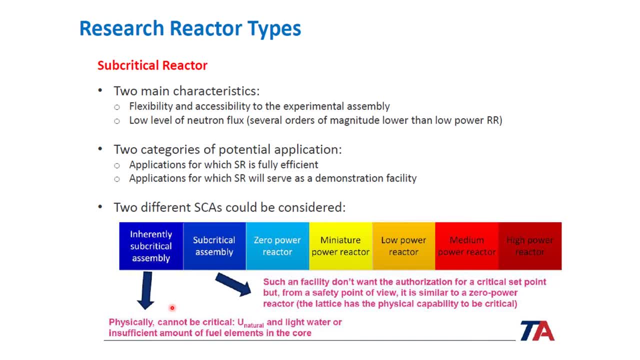 because the natural uranium and light water or insufficient amount of fuel elements in the core And the subcritical assembly, where such facility don't want the authorization for a critical set point. But from a safety point of view it is similar to a zero power reactor. 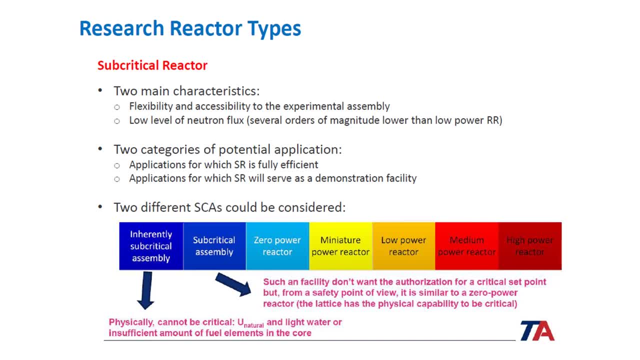 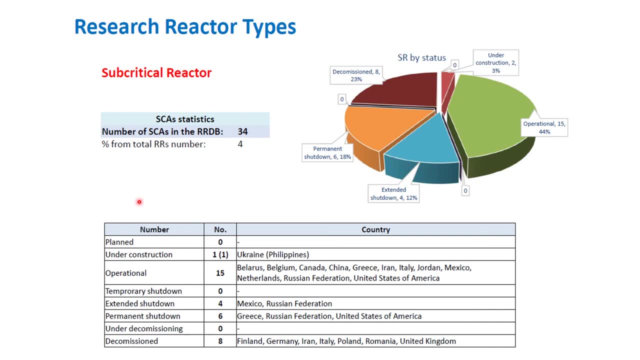 wherein the lattice has the physical capability to be critical. So these are the number of subcritical reactors around the world. So we have around 34.. So under construction or this one? this data here do not yet include the Philippines, But if you're going to include the Philippines, 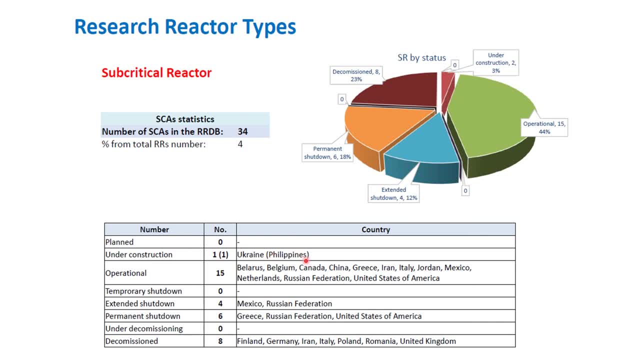 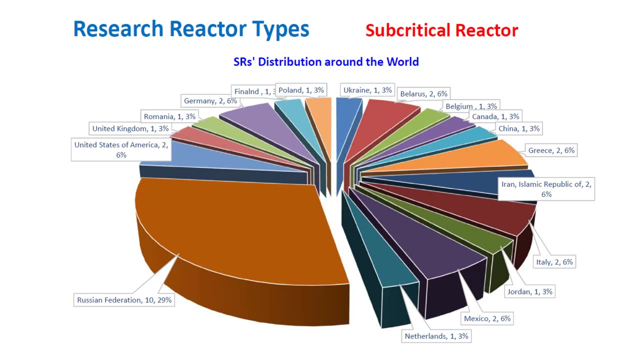 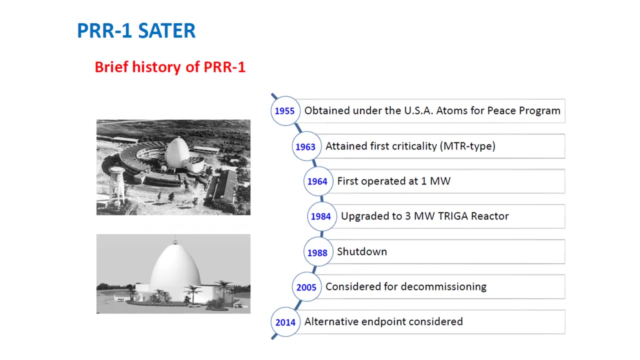 we have one which is under construction And you have 15 operational And we have eight that are the commission. So these are the subcritical reactors distribution around the world. Many of the SRs are located in the Russian Federation. The Philippines is actually not a newcomer. 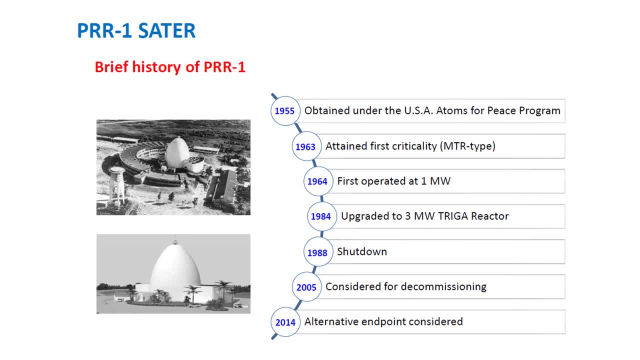 when it comes to research reactors- This is a brief history- We have your Philippine Research Reactor 1, wherein, in 1955, we obtained, under the USA Atoms for Peace Program, a project for a research reactor In 1963,. 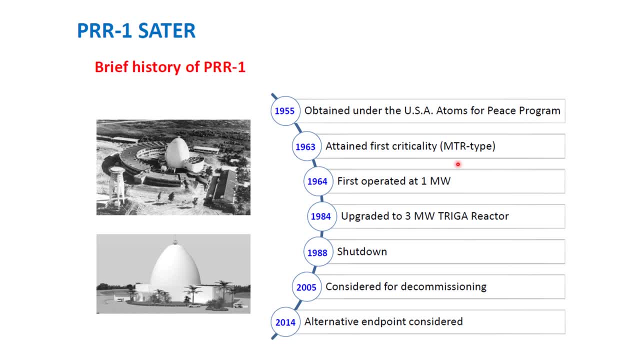 it attained its first criticality as a material testing reactor type And in 1964, it was first operated at one megawatts. From 1964 to 1984, for 20 years, it was used in various applications in research. 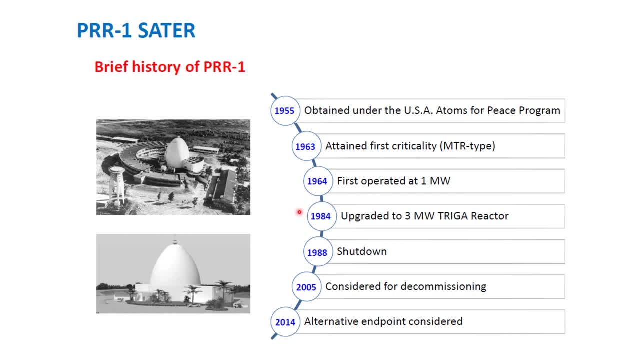 and also in training. And then in 1984, it was decided to be upgraded to three megawatts trigger reactor. The upgrading finished in 1988. And then it was initially found to be successful. However, after some weeks there were some issues found. 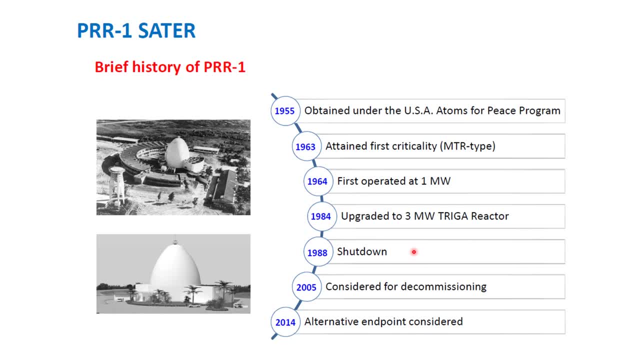 until it was decided that it will be for shutdown. So the issues were not fixed until 2005,, wherein the PRR-1 was considered for the commissioning. However, in 2014, there was an alternative endpoint considered for PRR-1. 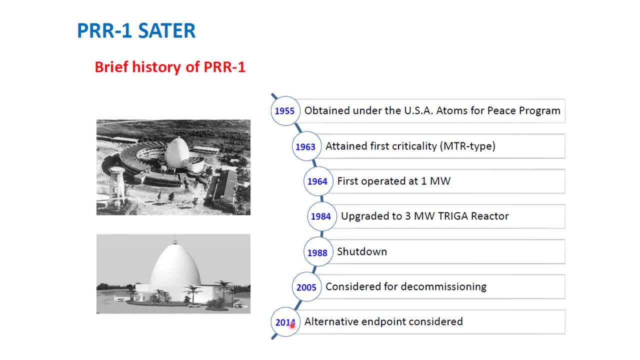 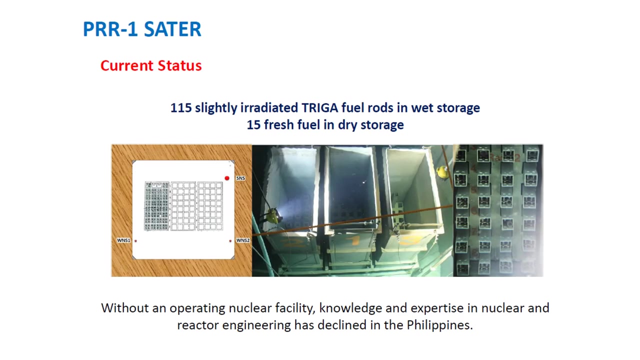 as not to waste the unspent nuclear fuel. So this one here, as you can see, is an egg-shaped structure. This is where your PRR-1 is located, And this is still very much present today in the Philippine Nuclear Research Institute. 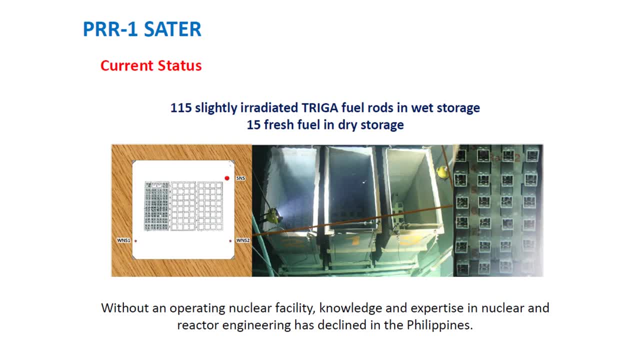 So, for the current status, we have 115 slightly radiated trigger fuel rods in wet storage and 15 fresh fuel in dry storage. So this is the reason why, in 2014,, there was an alternative plan for your PRR-1, instead of it being the commission. 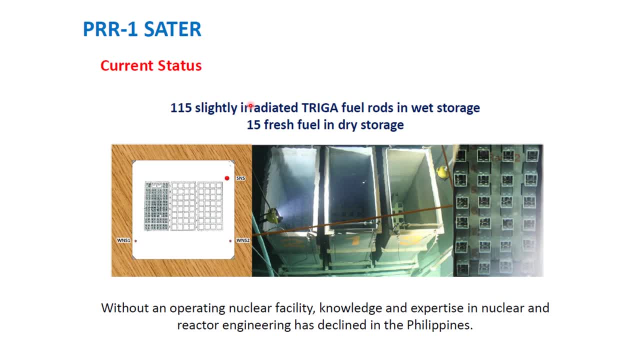 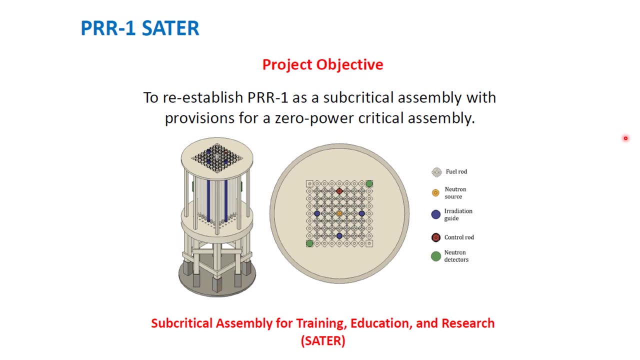 So without an operator operating the nuclear facility for more than 30 years, knowledge and expertise in nuclear and reactor engineering has declined in the Philippines. The objective of PRR-1 SATR is to establish PRR-1 as a subcritical assembly with provisions for zero-power critical assembly. 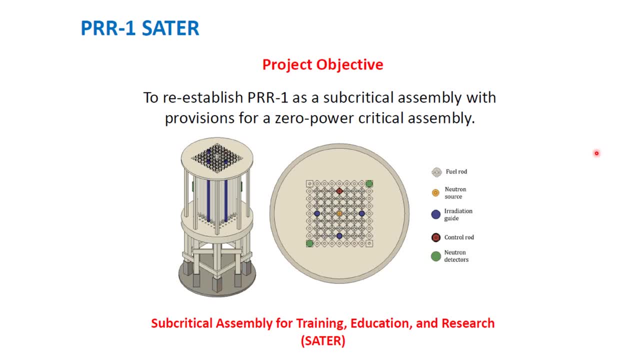 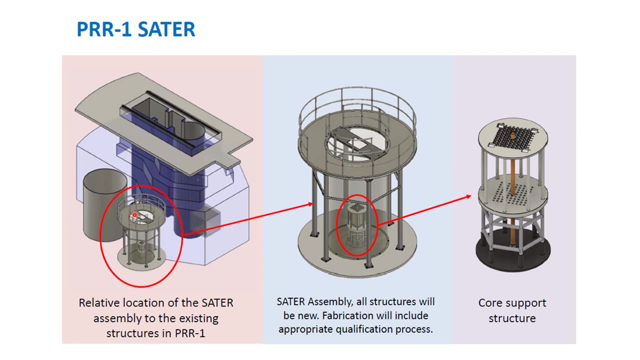 So SATR stands for Subcritical Assembly for Training, Education and Research. So that is SATR And this is the relativization of SATR assembly with respect to the existing structures of PRR-1.. And the SATR assembly. 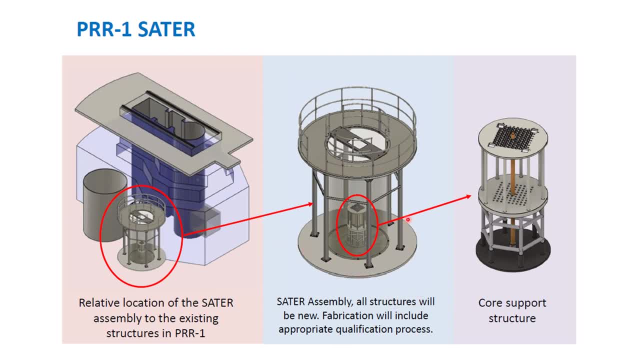 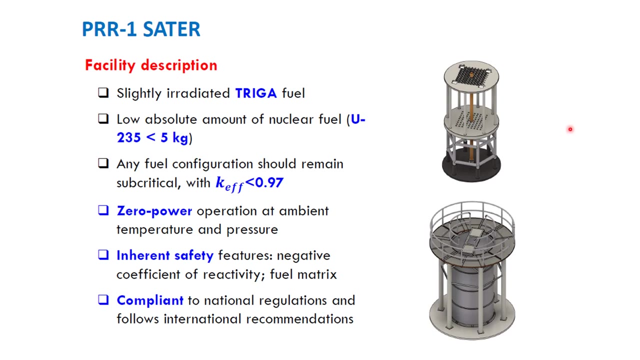 all the structures will be new and fabrication will include appropriate qualification processes, Including new core support structure. This facility description for your PRR-1 SATR. it is slightly irrigated or it will use slightly irrigated trigger fuel in order to avoid more nuclear waste. 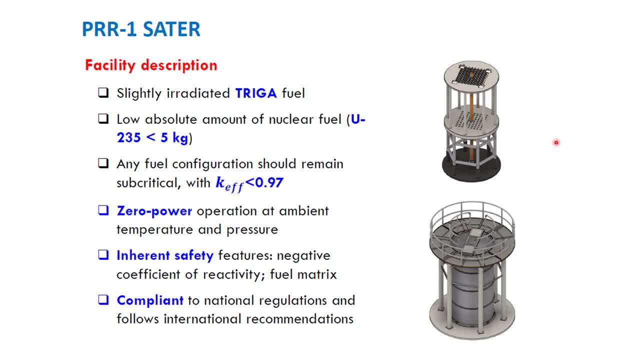 by using a new fuel. It has low absolute amount of nuclear fuel. your uranium-235, less than 5 kilograms And any fuel configuration should remain subcritical with coefficient of less than 0.97.. Zero-power operation at ambient temperature and pressure. 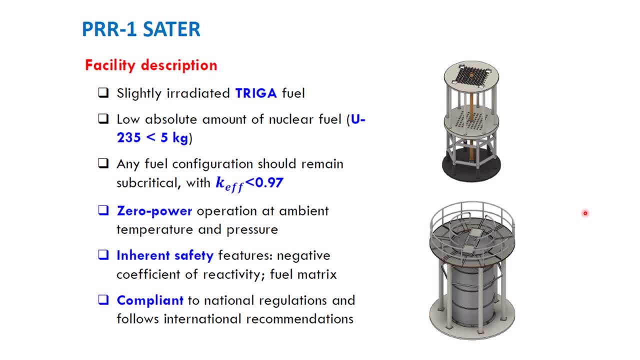 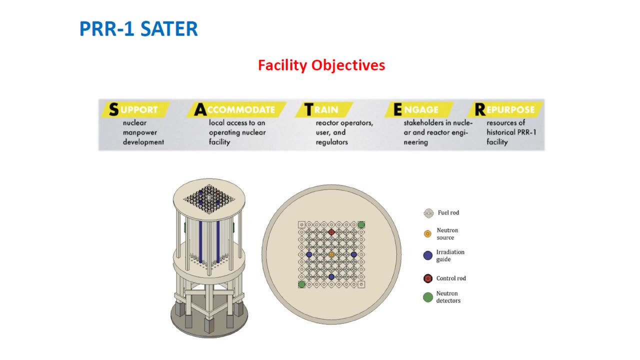 and inherently safety pressures because of the negative coefficient of reactivity and the fuel matrix. And it will also be compliant to national regulations and follow international recommendations. These are the facility objectives of SATR: To support, accommodate, train, engage and repurpose. 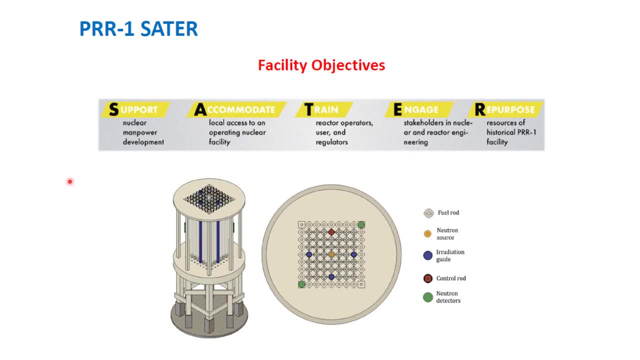 Support nuclear manpower development, which is very timely- Timely because of the signing of Executive Order 116, which we are going to discuss in the next session, And to accommodate local access to operating nuclear facility, To train reactor operators, users and regulators. To engage stakeholders. 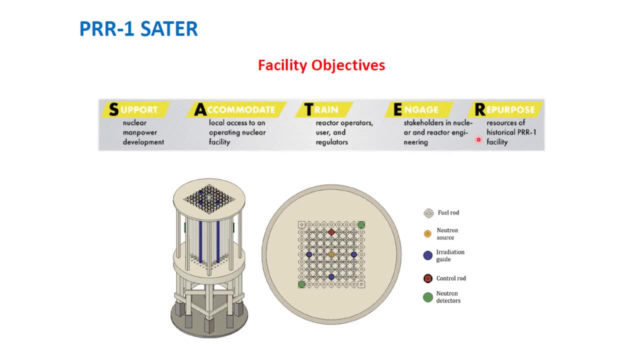 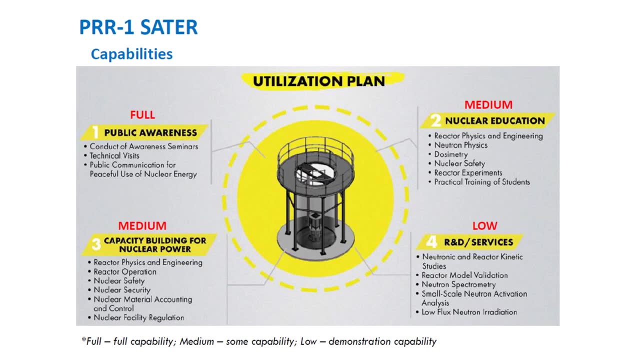 in nuclear and reactor engineering And to repurpose resources of historical PR-01 facility that were not used. This is the utilization plan of the PR-01 SATR capabilities. We have full utilization for public awareness, to conduct awareness or seminars, technical visits and public communication. 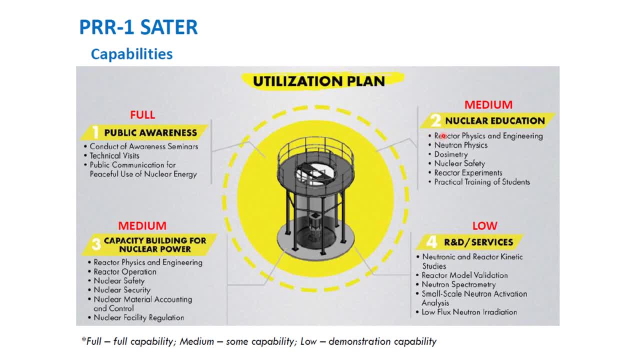 for peaceful use of nuclear energy. We will have medium utilization for nuclear education in reactor physics and engineering, nuclear physics, the cemetery, nuclear safety, reactor experiments and practical training of students, And also medium utilization plan for capacity building for nuclear power, For reactor physics and engineering.